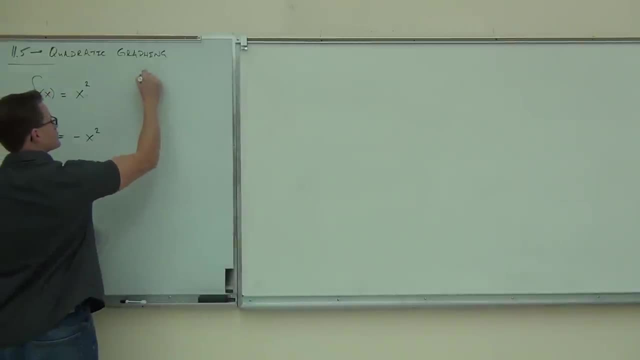 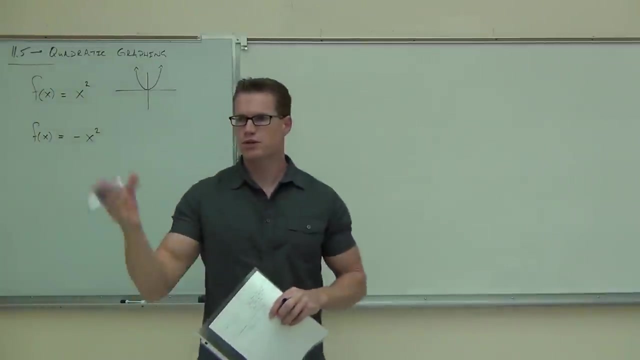 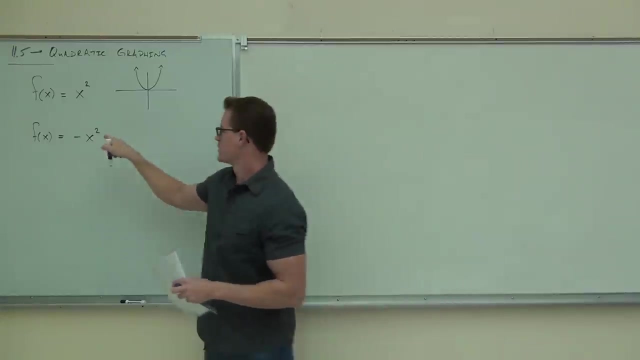 remember that This one looked like this: A nice U-shaped graph going from the origin upwards at a nice curving slope. Are you guys with me on that? What did this one look like? Ah, so this right here, that negative flipped this or reflected that across the. 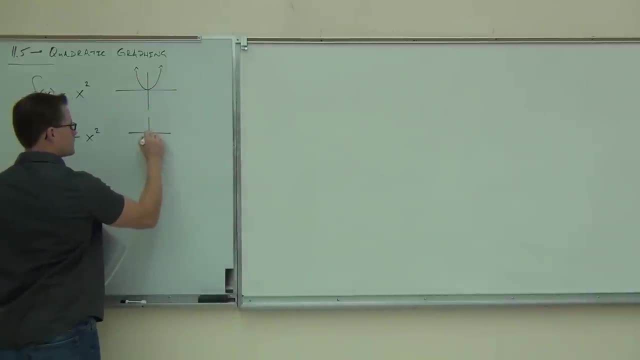 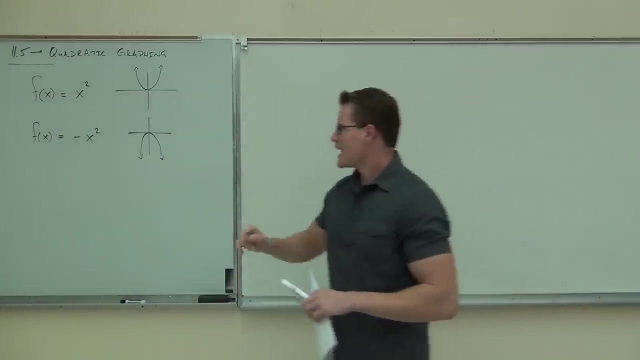 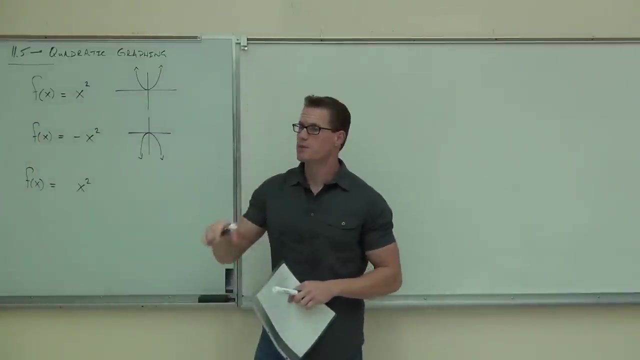 x-axis. yeah, Pretty much the same looking graph, though, right? Well, here's the deal. Anytime we have a graph that has an x squared in it where the square is the largest power, so, for instance, This right here: Anytime we see that square, that means you are going to be dealing with. 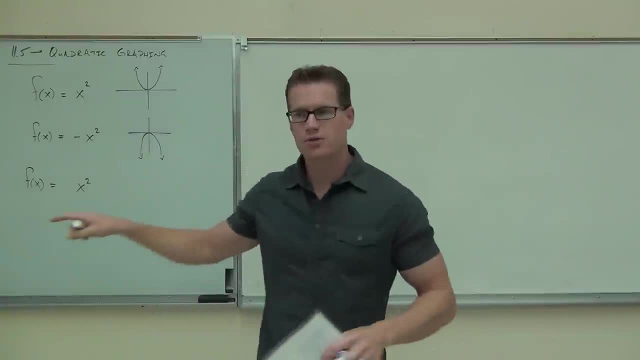 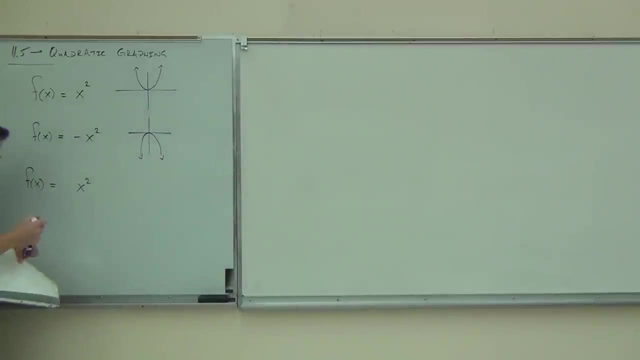 a parabola, because you've got a quadratic function, This right here. when we have this equal to a function, that's called function notation. So this is a quadratic function And, in general, here's what we can do with that. We can say that anything that looks. 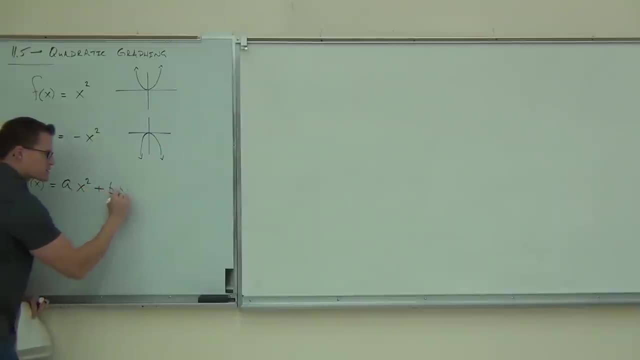 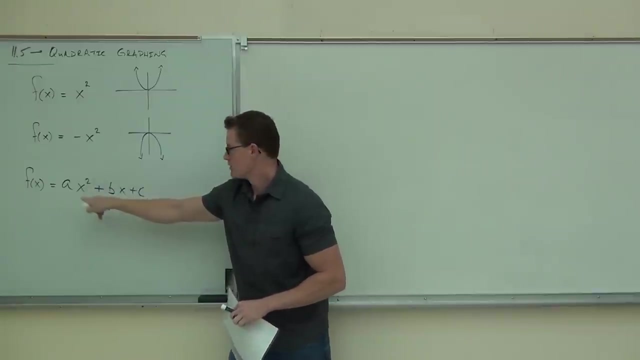 like this, with an ax squared plus bx plus c, anything of this form where that x squared should stand out to you. Does that stand out to you? Yeah, Because I have it in a different color. Of course it stands out to you. 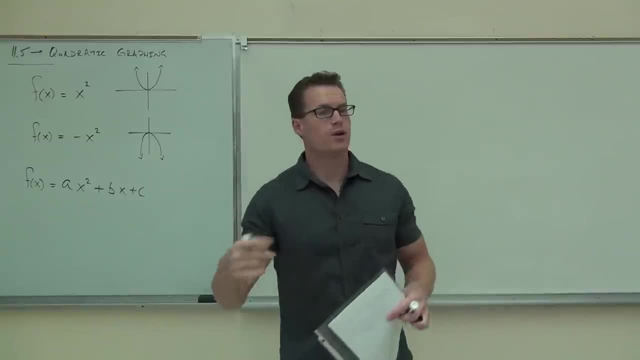 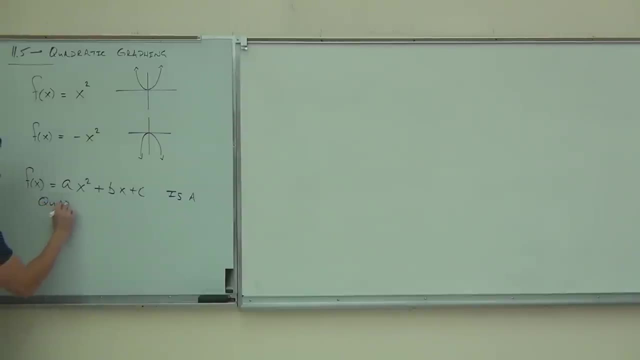 But anything with that square, that is a parabola That we're going to be able to graph. So this right here is a quadratic function. Clearly quadratic because it's of that quadratic form, Clearly a function because we have it in function notation. 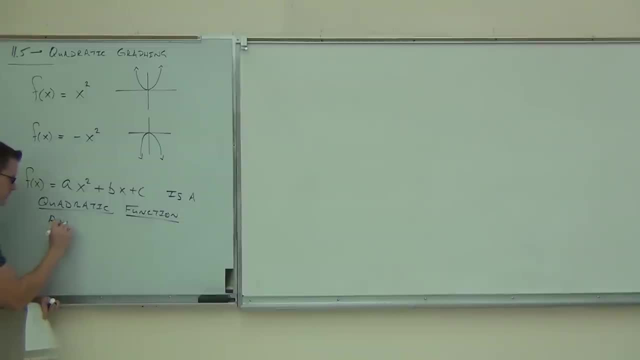 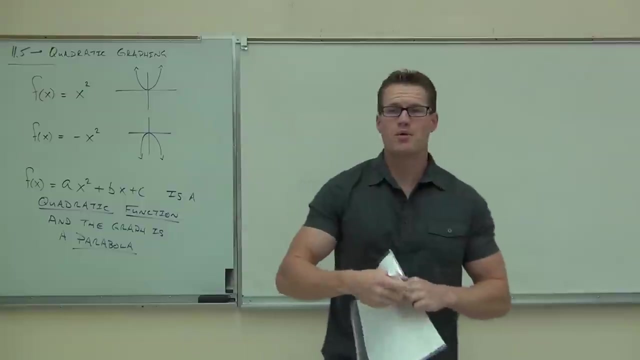 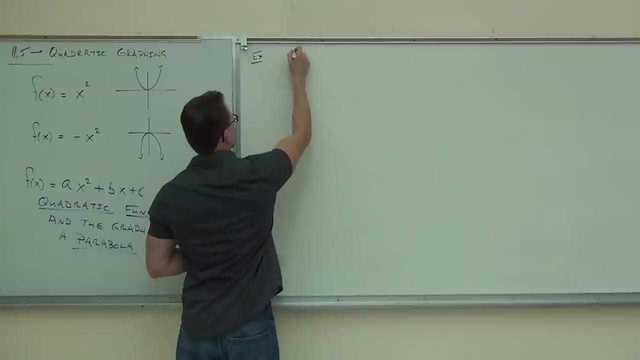 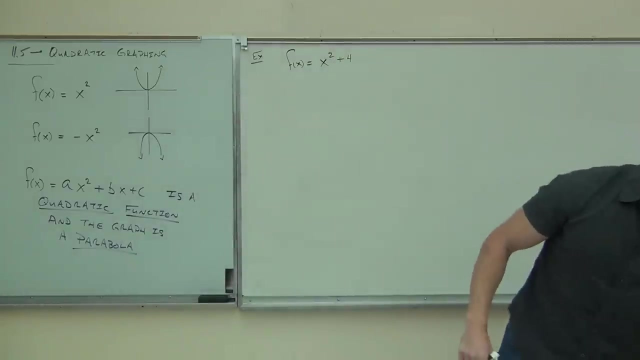 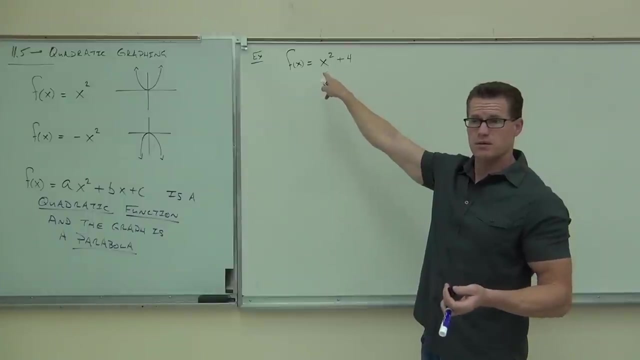 And the graph will be a parabola. Now let's see if you remember back to chapter 8 stuff. Firstly, ladies and gentlemen, look up the board with me. Is this a quadratic function? Does it have an x squared? Does it have a function? 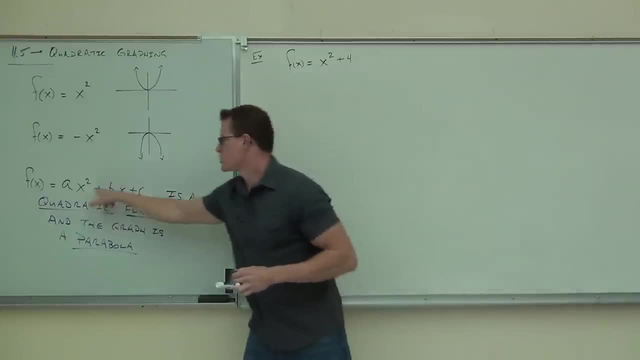 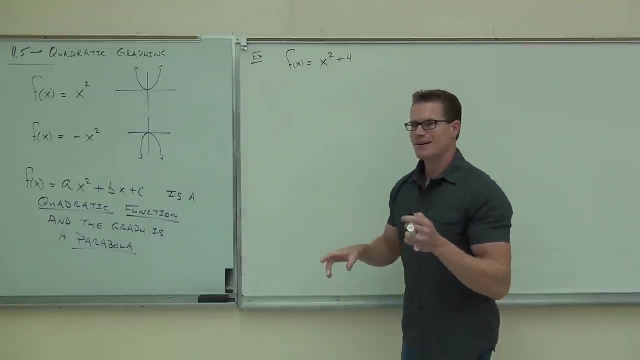 That's a quadratic function. It doesn't matter if it has all this other junk, okay, As long as it has an x squared, that automatically qualifies it as a quadratic function. You with me? Hey, hey, hey. Does this still make a parabola? 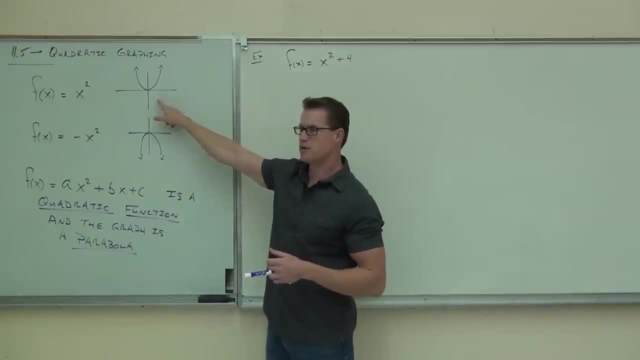 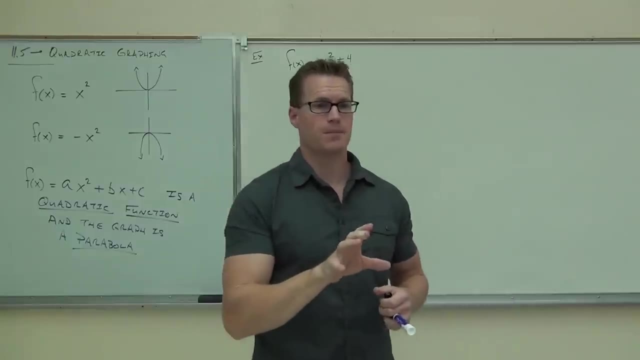 Is this parabola going to be exactly like this one? What's the difference between this and this? That plus 4 did something. Now that plus 4, you need to tell me whether it moved it up, down, left or right. 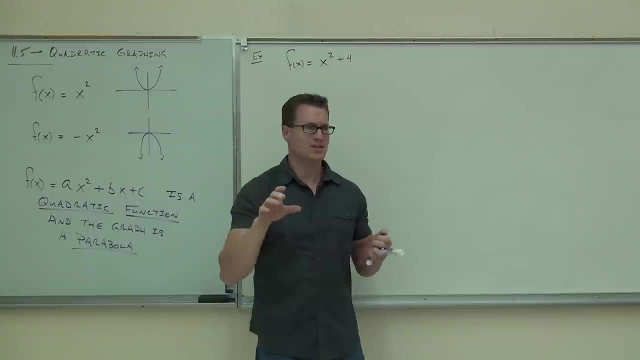 Left. I said some people say left, some people say up. One of you is right. Oh, try up, because it's not inside the, It's not in parentheses, is it? This says you're going to do a whole bunch of stuff to this, and then, at the very end, you're going to add 4, which says move it up 4.. 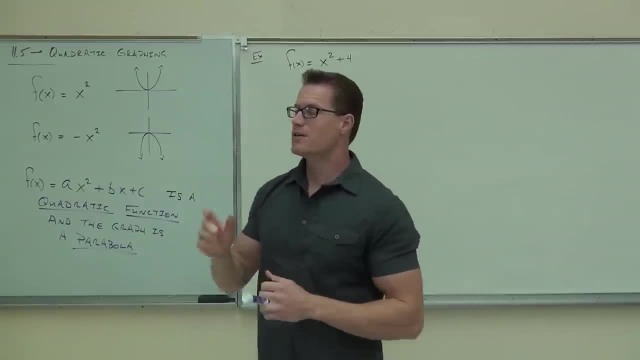 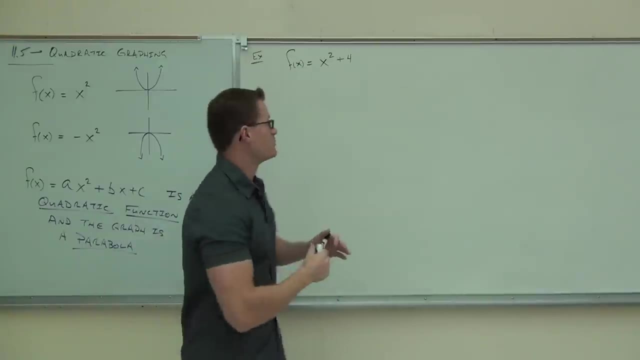 Do you remember that? Yeah, This right here is a shift up 4.. In fact, any time, Any time. Let's go back to chapter 8.. This is our basic graph shapes, right? Any time you have a plus or minus at the end of your function, that is, shifting your graph up or down, right? 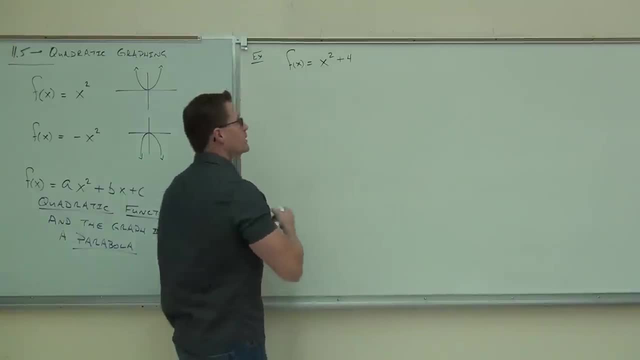 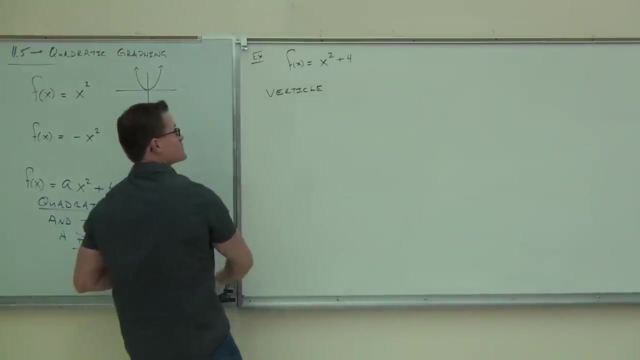 Plus means up, minus means down, So we're going to talk again about vertical shifts. Maybe that shift was going to come back at you, right? Thanks for the courtesy, lad. I think I even misspelled vertical. I was too involved in my own joke. 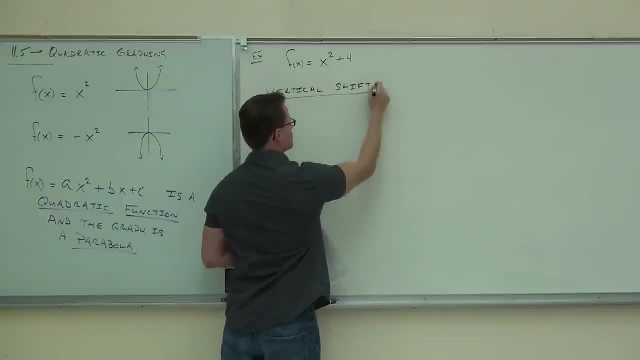 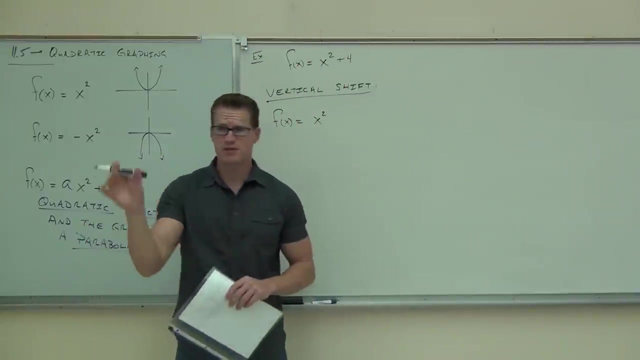 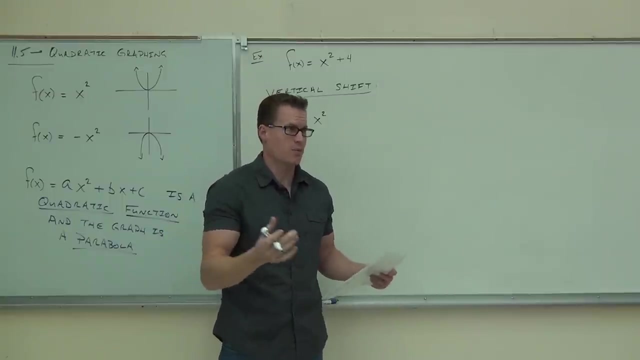 Vertical shifts. So if we have x squared, this is what's going to be kind of nice about this section. It is exactly the same as the chapter 8 stuff, all that shifting. So if you remember the shifting you are ahead of the game. except we don't have any other shapes to remember except the parabola. 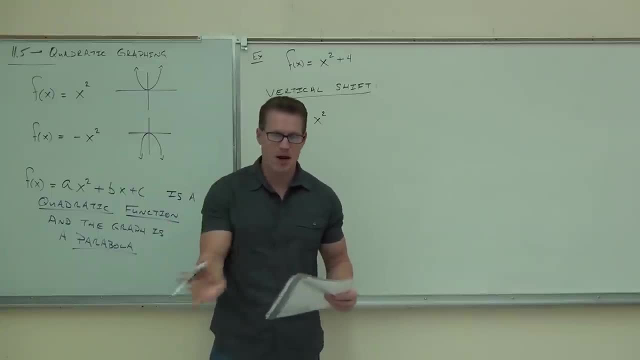 So what are we going to be graphing every single time? Parabola, Parabola. If you have anything besides a parabola, are you doing it right? No, No straight lines, no v's, no weird curves, just parabolas. 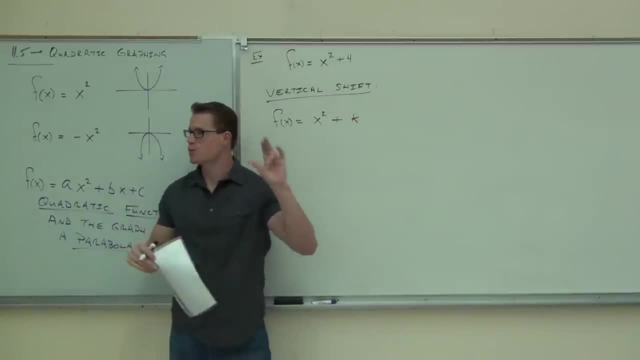 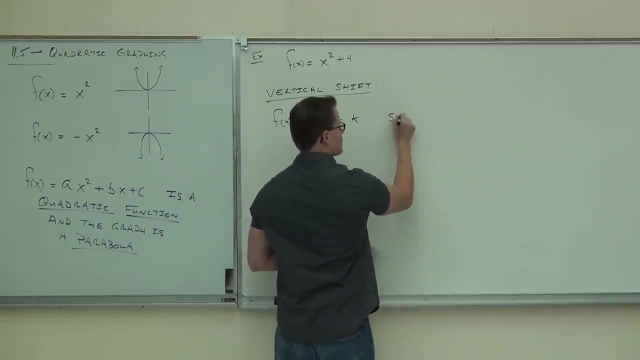 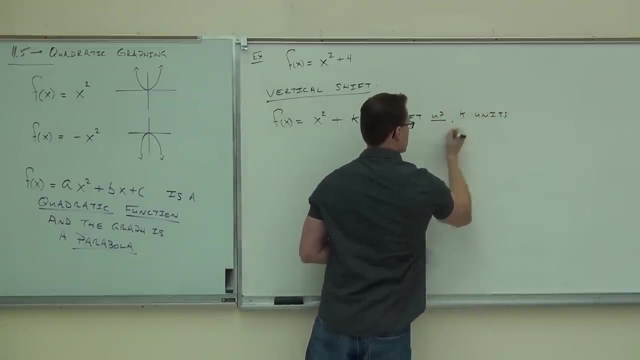 If we have x squared plus k, so some parabola plus k. what that's doing is that's shifting it. what was it again? up or down Up? This is up k units. This is a shift up K units. 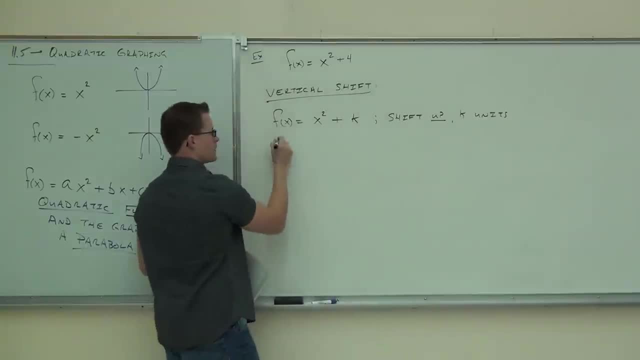 K units, Which means that if we have x squared minus k, well that's just going to be a shift down k units. So we're taking this graph right here, our basic graph shape from chapter 8, the x squared. that's a parabola starting at the origin and we're just shifting it up or down. 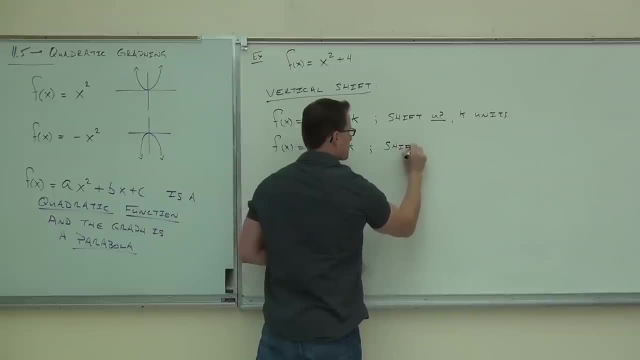 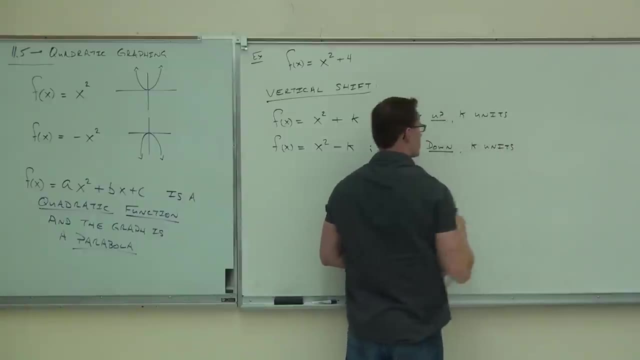 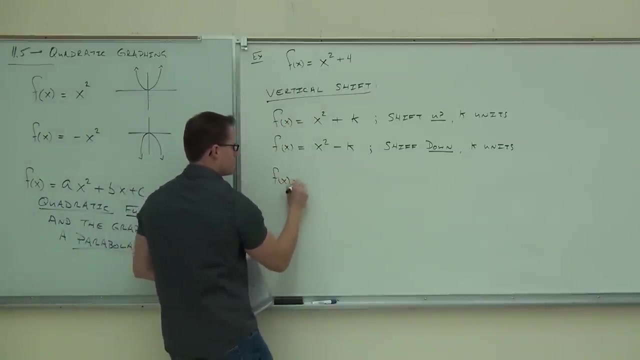 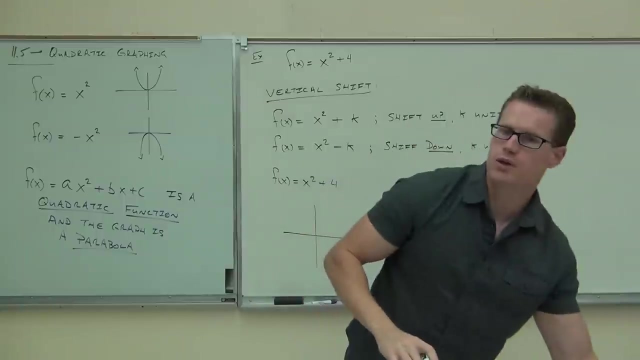 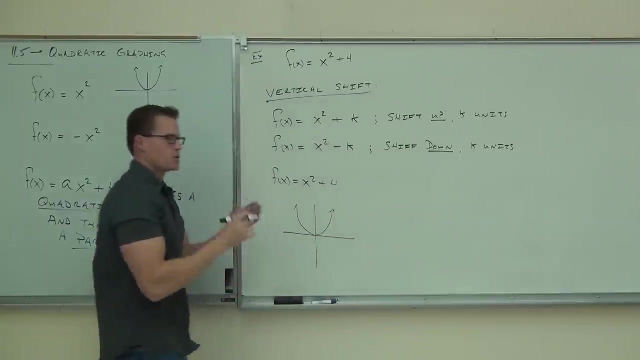 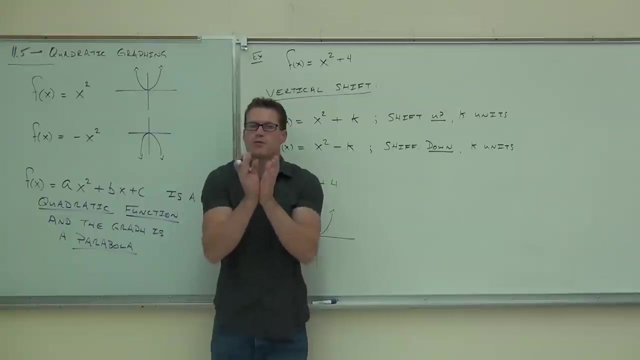 shift this. this says plus 4, that means on the vertical we're going to shift up 4 units. 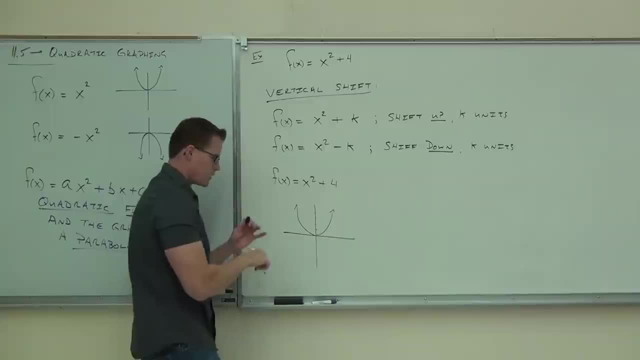 That says, we move up 1,, 2,, 3, 4 spots. We'll redraw the exact same graph and we'll label it. though You've got to label it. if you're going to draw two of them, Do you have to? 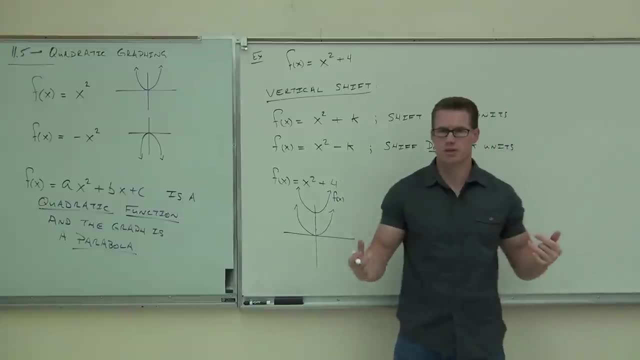 draw two of them. No, I don't care anymore, But you need to know what your original one looks like. Your original graph looks like this parabola, this basic graph shape that's on the board. We've shifted it up 4 units. That is the graph that we just drew, that. 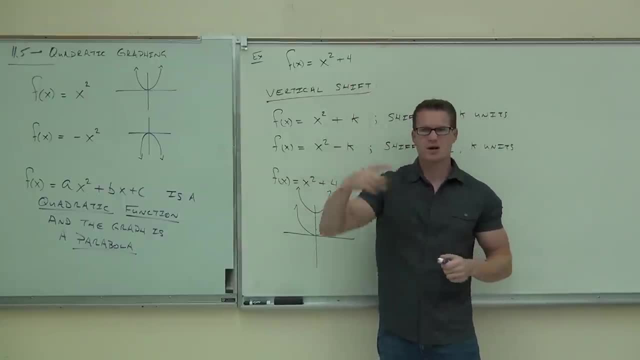 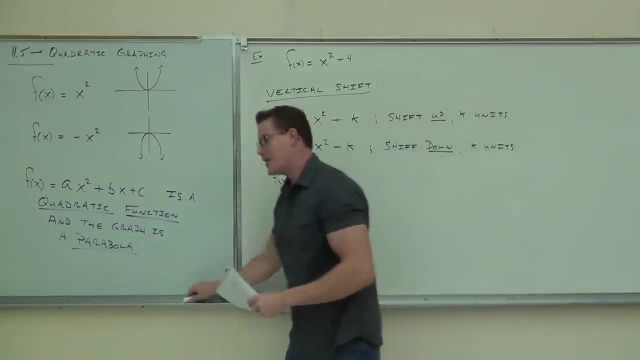 function x squared plus 4.. Raise your hand if you feel okay with this. Is this coming back to you? I hope so. This is your second shot at it, right? So if you didn't really master this concept in chapter 8, this is it again Now. we should just hammer it. 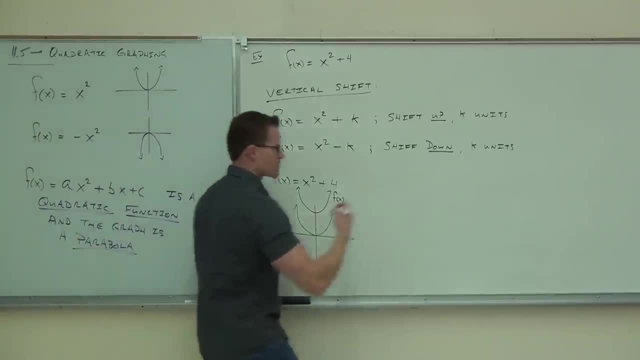 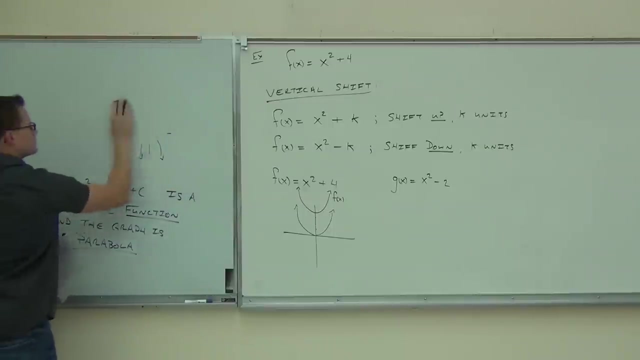 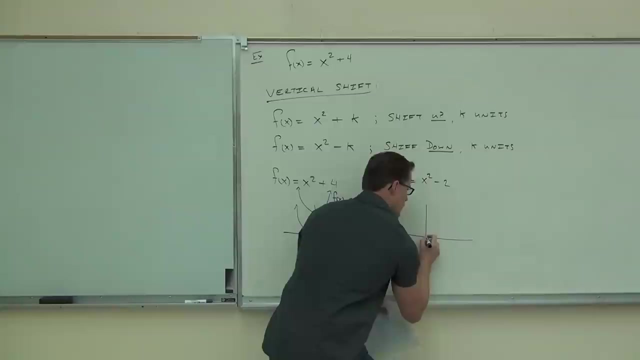 Why don't you try one of your own, just to make sure that you can do it? Just grab that for me. g of x equals x squared plus 4.. Again, what's nice about this section? we're always starting with our basic x squared and. 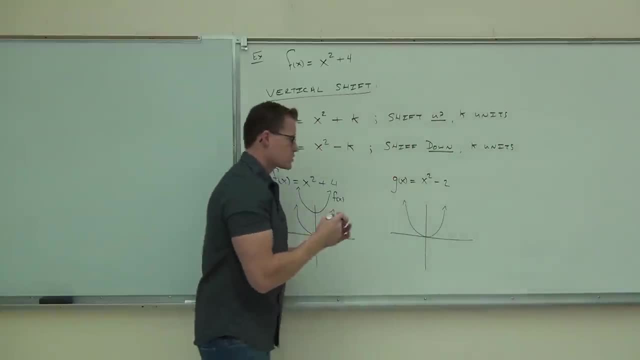 it's going to be shifting that around. That's all we're dealing with in this whole section. This shift is this: up down, left or right? This is going to be shifting that around. This is going to be shifting that around. This is going to be shifting that around. 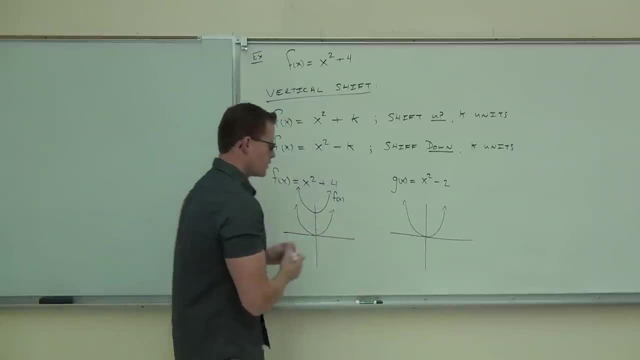 What do you think? Down, Down, how many? 2. So we go down 2. That means we're moving pretty much our vertex. This lowest point, or highest point in the case we've got over here, is called your vertex. We're just really. 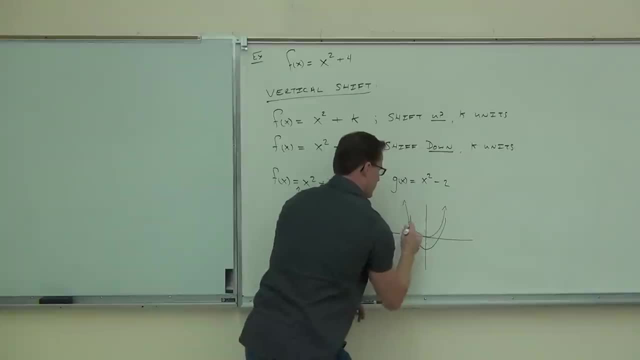 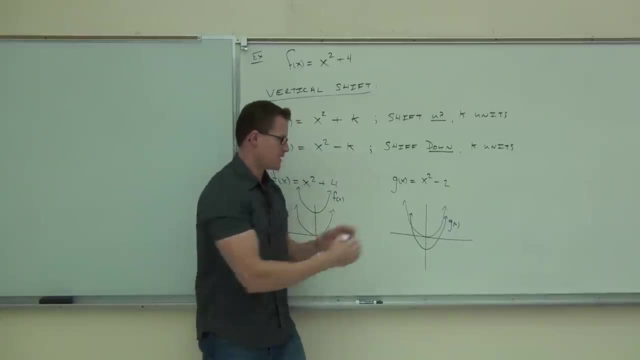 shifting that and redrawing our graph. That's about right, And we'll label that so that we know what graph we have. I made mine too skinny, but that's okay. It lost some weight. Now how about this one? Was that still a shift down? 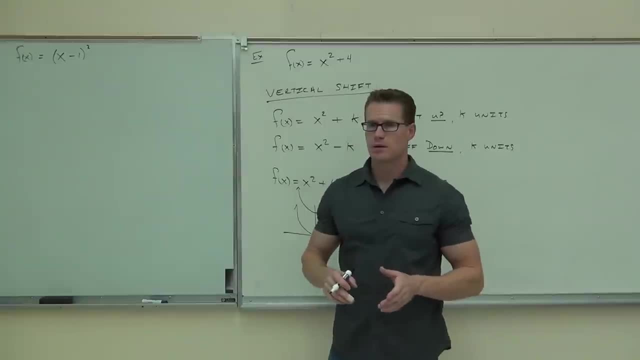 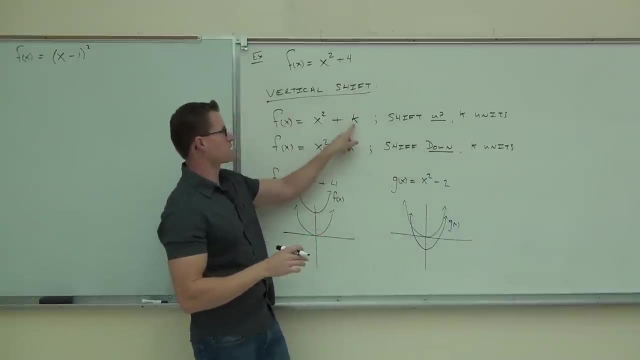 No, Was that still a shift up? No, So is this a vertical shift at all? No, Vertical shifts come at the very end of our problem, end of our function. This right here, this plus k, this minus k, that's after everything's been done. right, It says: you do all this stuff. 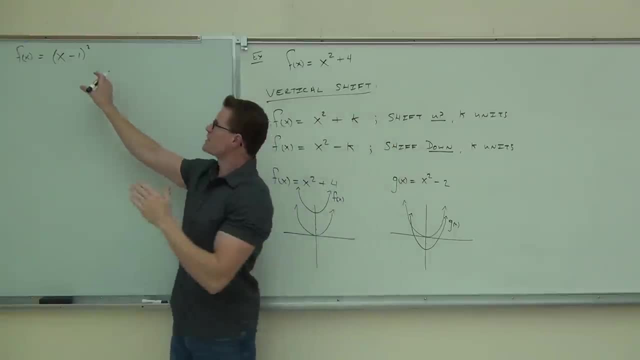 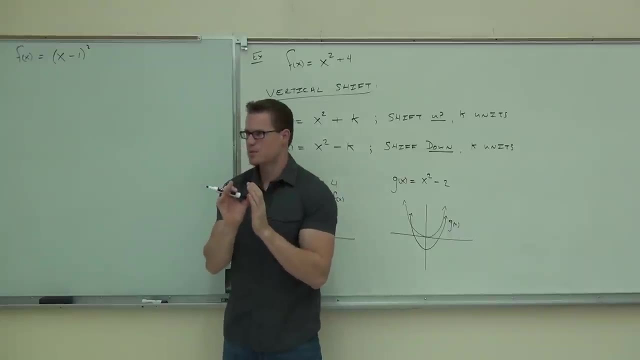 and then you're moving it up or down a little bit. That's what's happening here. This one, that's within the function, says I'm either speeding up or I'm slowing down. my function That's moving it either left or right like a timeline. Remember talking about the timeline. 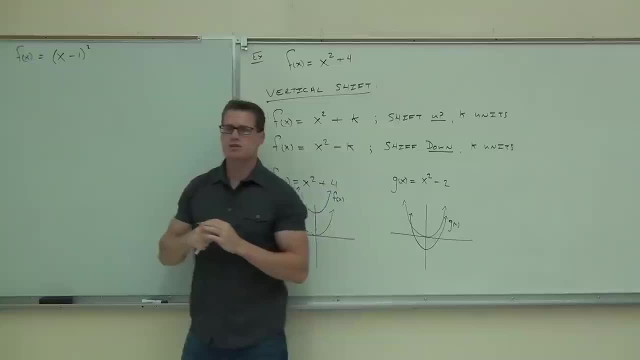 idea. This right here. this slows down our function. So whatever number we plug in, we take away 1 from it. So instead of starting here, it's starting later. Later is part. like, if you want to think of it as a timeline, It's starting numerically later. So if I plugged 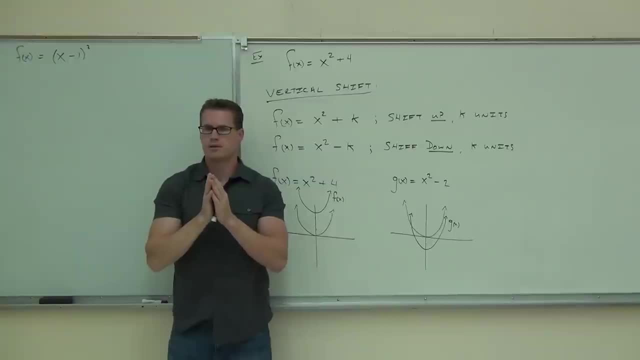 in 2, it'd be like I was plugging in 1 for that value. So it's actually slowing it down. It's saying if you started here now, you're starting a little bit later. So is this going to be a left or a right shift? 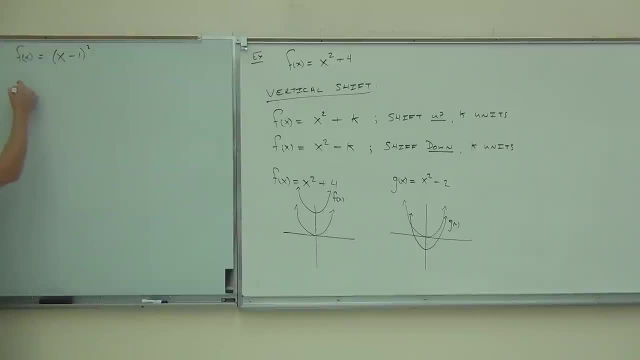 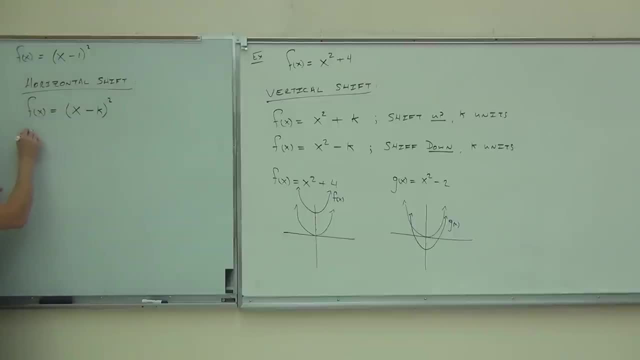 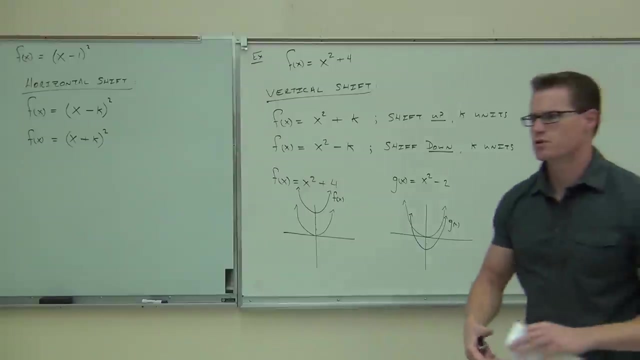 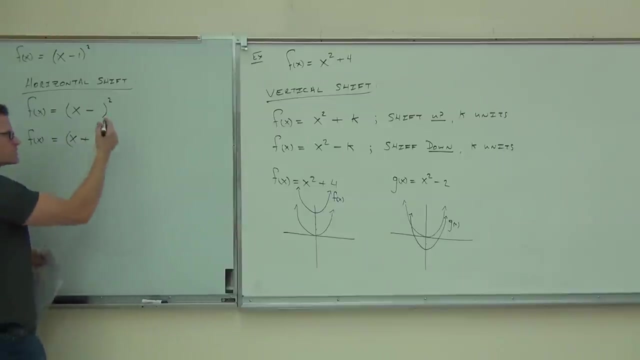 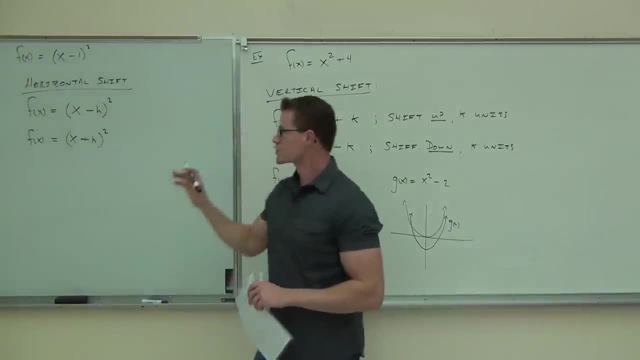 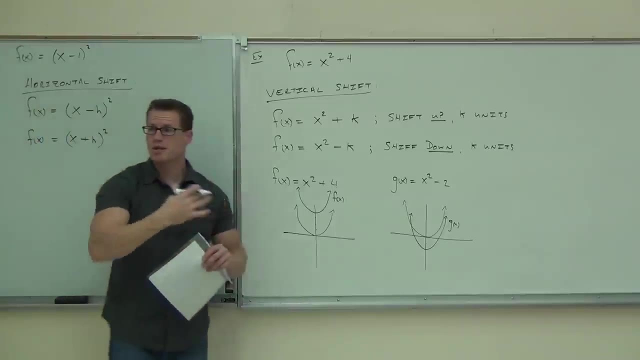 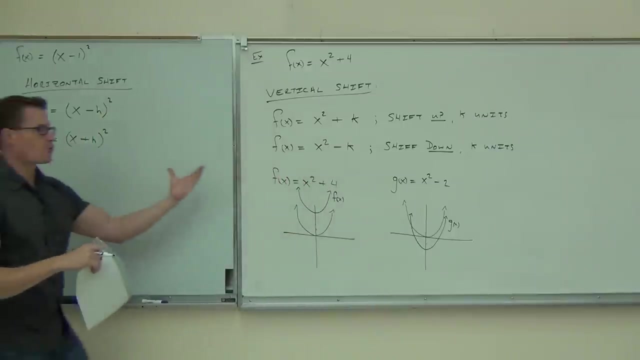 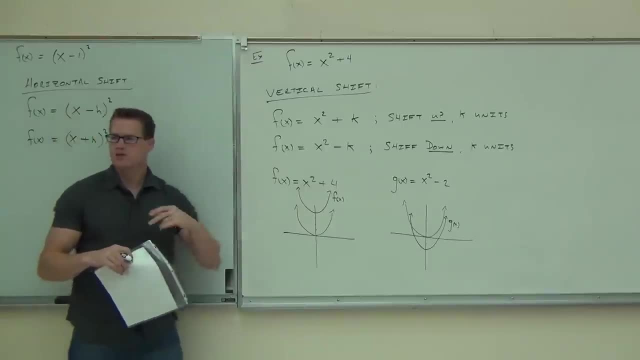 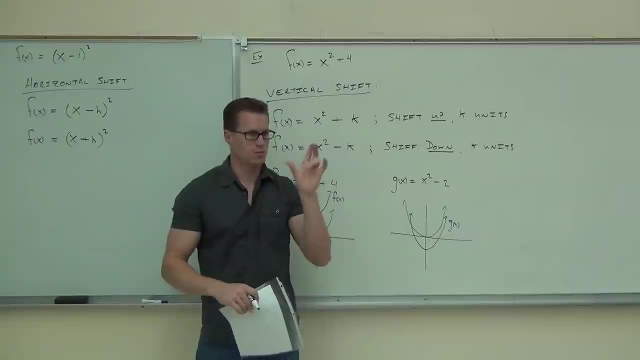 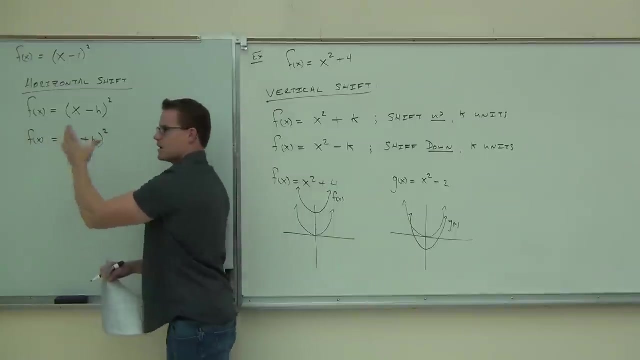 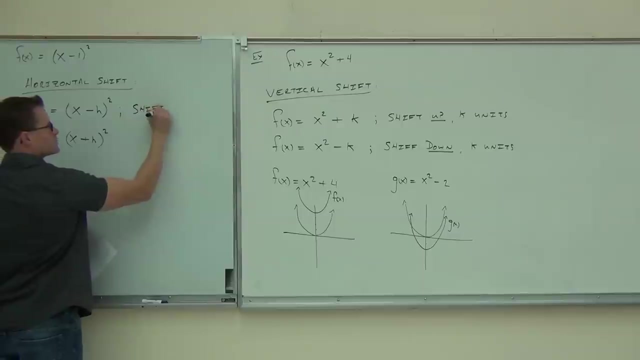 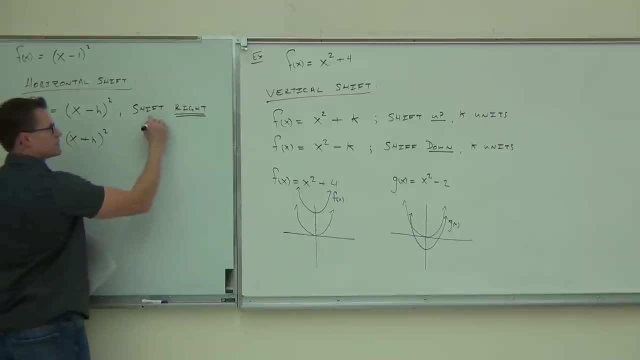 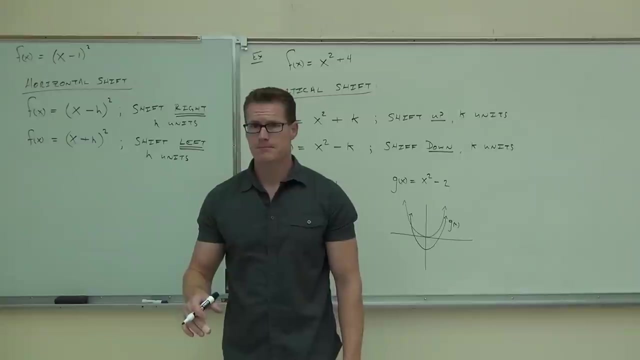 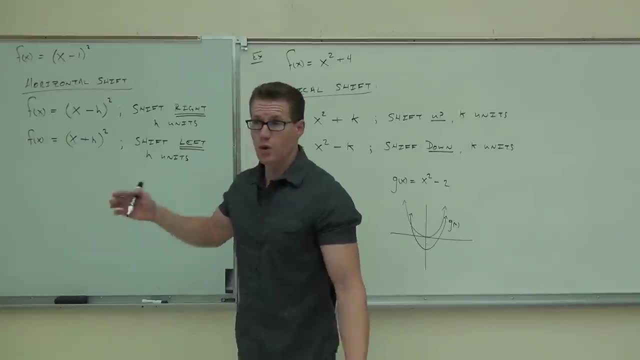 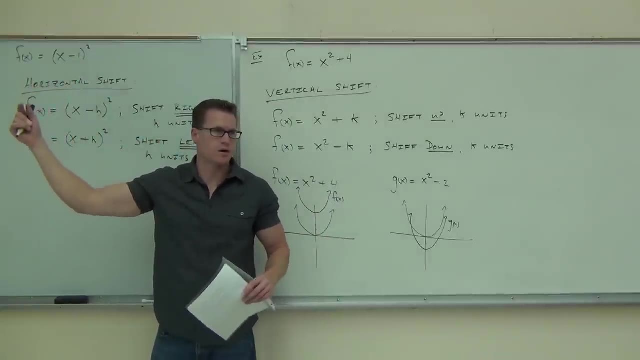 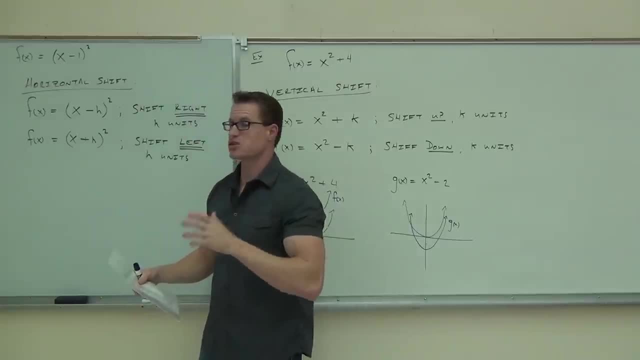 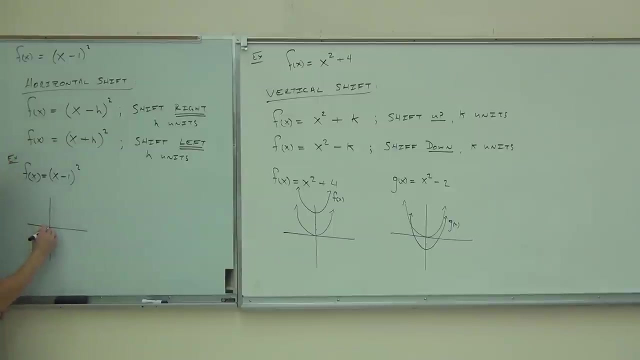 So we're just going to be shifting things around. That's what this section does for us. So let's go back to this problem. We'll go ahead and graph that. So, again, what we're doing is we're starting with our original graph. 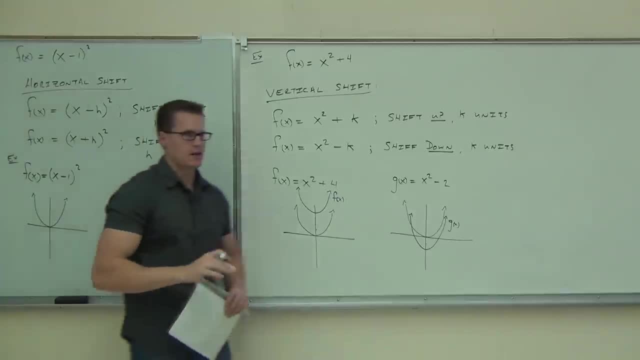 That's just a nice x squared graph, And then we're going to be shifting it. In this case, this said, we're subtracting 1 from our number before we square it. That's going to slow down our graph. So instead of starting right here on the y-axis, we're starting a little bit later. 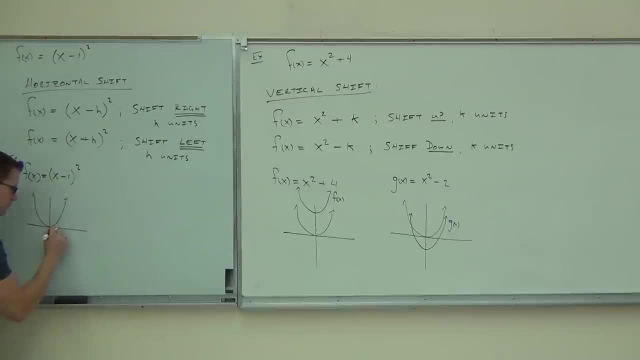 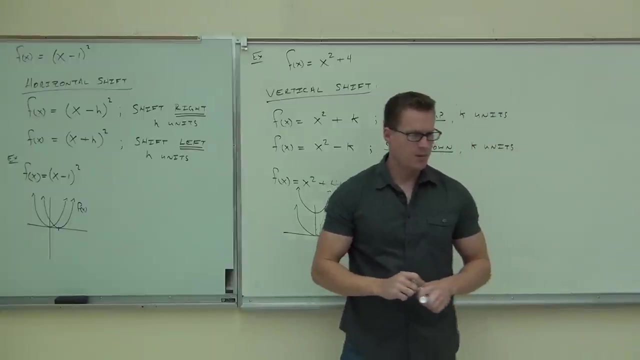 So we're shifting it to the right one spot Again. we're shifting the vertex over. We'll redraw it. That's our graph. How many people feel Okay with this one so far? Yes, no, All right, Let's try one here. 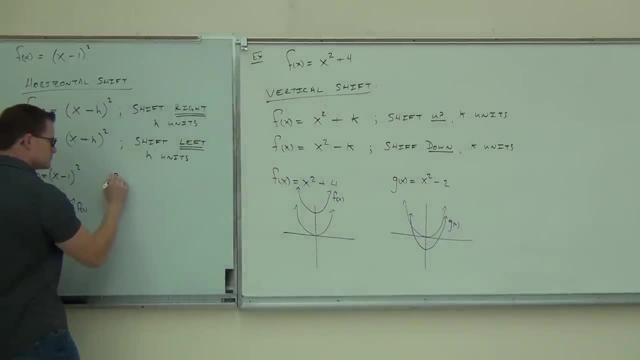 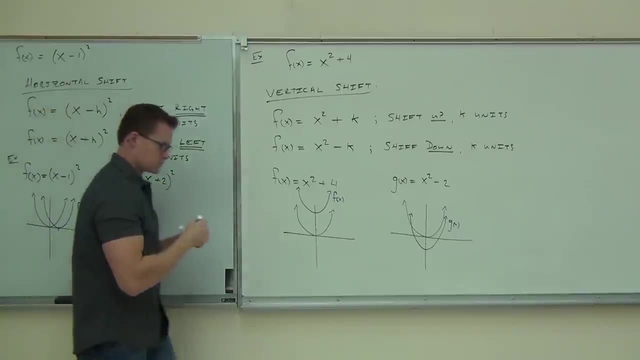 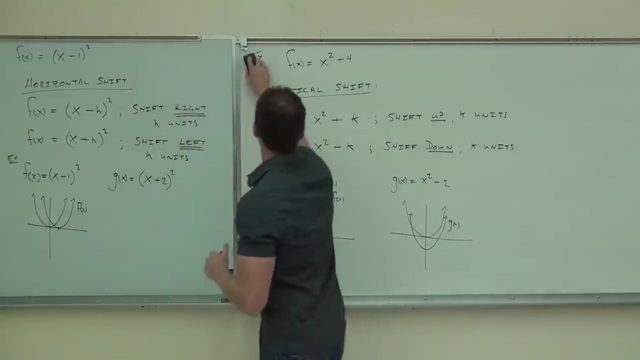 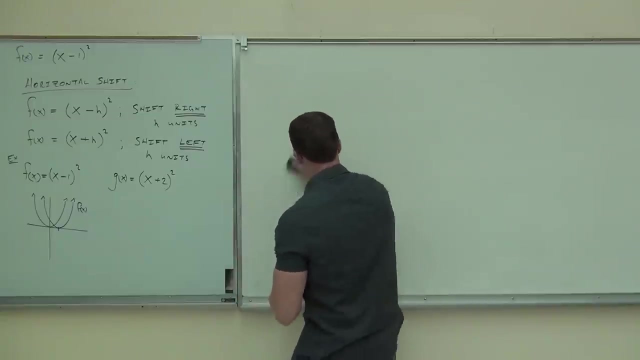 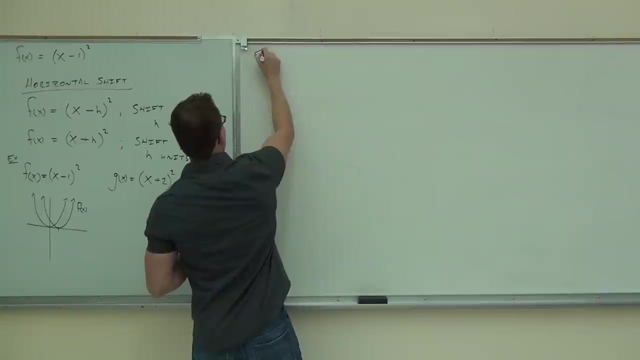 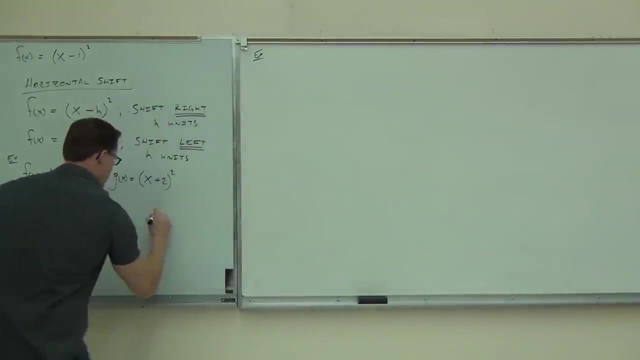 Oh, we'll keep going. Go ahead and graph that one Do. the g of x equals x squared plus 2.. So we start with our original x squared. You can choose to draw that or not. Honestly, it really doesn't matter. 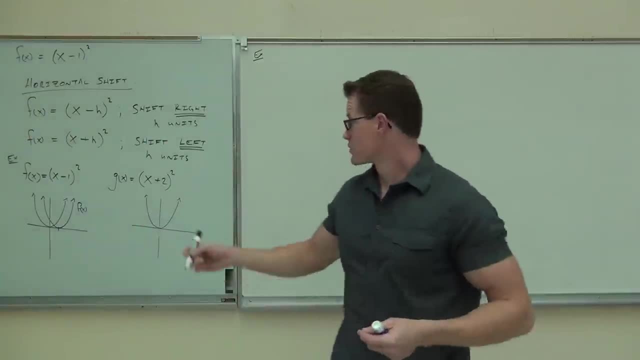 We just need to have the shifting correct and label your graphs. So on this one, it is moving left, right up down. Which one Left Left? How many spots? Two, Good, So really we're just redrawing our parabola. 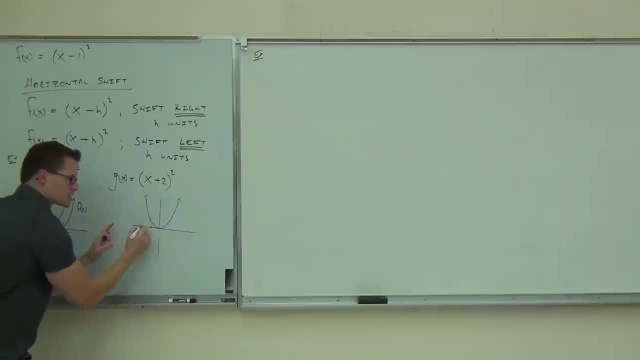 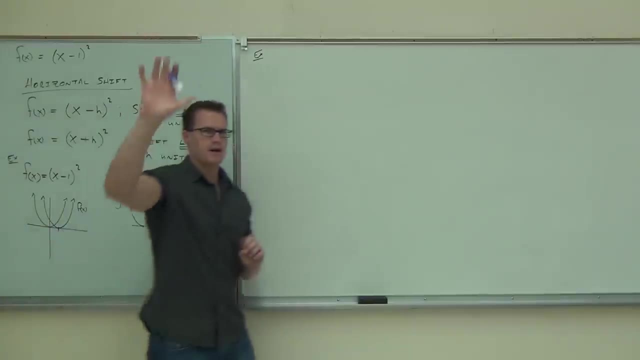 We're going to move it to the left two spots, And when I say it I mean the vertex. We'll redraw that. We'll be sure to label it. In this case it's g of x. How many people got that exact graph in their paper? 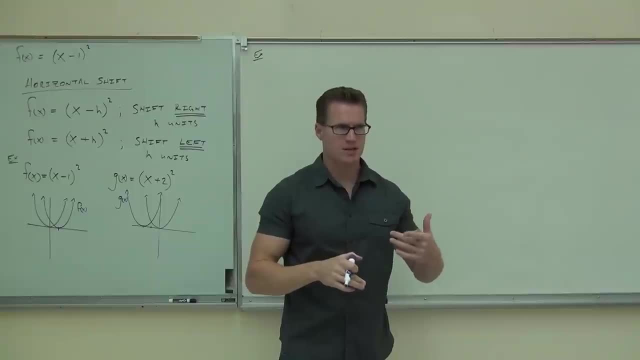 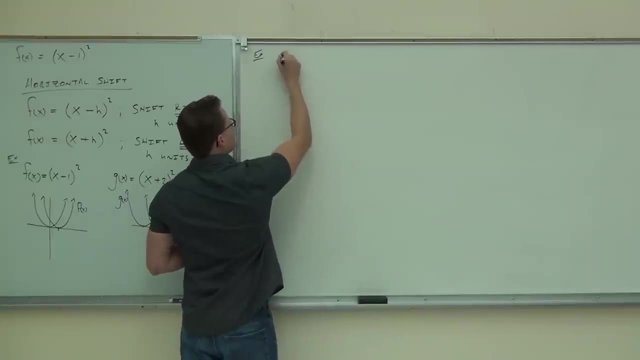 Okay, Are you starting to see how similar this is to the Chapter 8 stuff? Very, very, very similar as far as that shifting goes. By the way, did the letter go to the left? No, No, No, No. 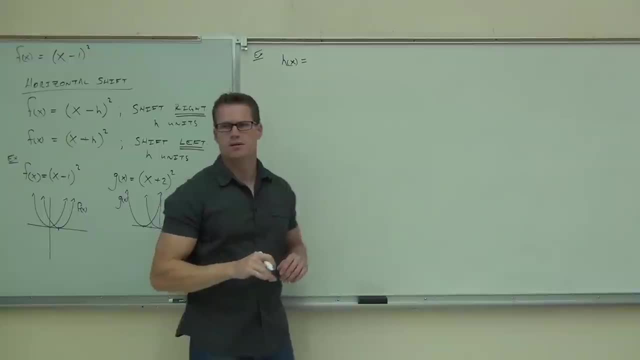 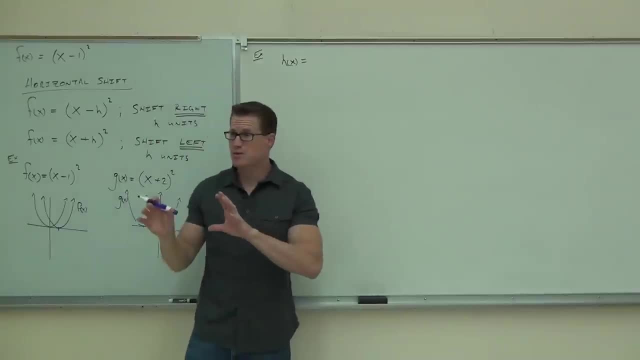 Every graph has a different name typically, And we have those different names because if we have to graph them on the same graph, we want to be able to identify between them. That's all that letter is doing. Can the shifts be combined? 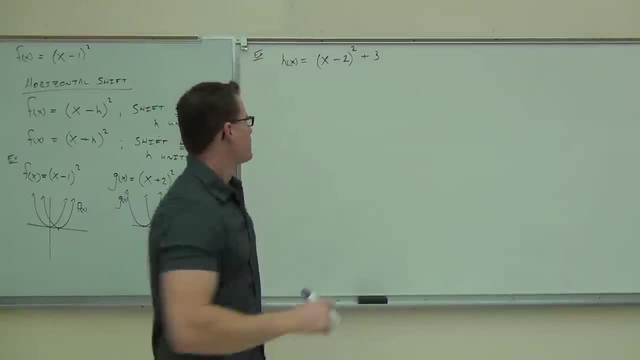 Yes, Yeah, absolutely. We did that last time too. We did that in Chapter 8.. So, really, we just need to be able to identify, from right to left, what's going on. So what does that plus 3 do for us? 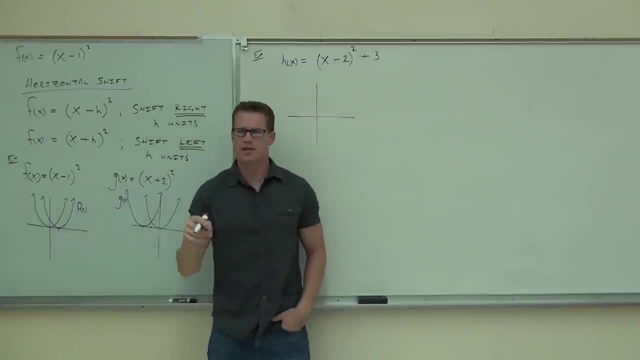 Is that a vertical or a horizontal shift? What do you think? Vertical, Vertical, Definitely. Is that going to be up 3 or down 3? Up Up. So we're going to circle that, just like we did last time. 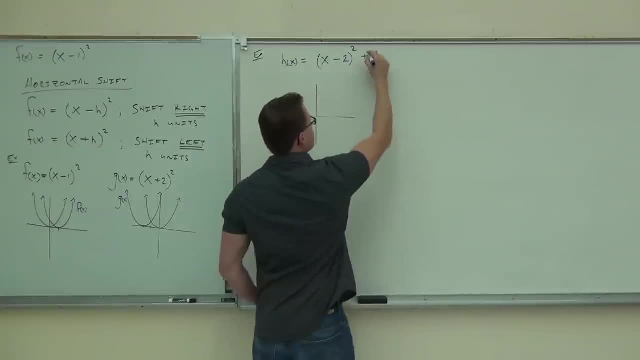 We'll say, okay, well, I know this is up 3 spots. This tells you you've got a parabola going on. That's kind of nice. What does this minus 2 do for you inside of our function there? 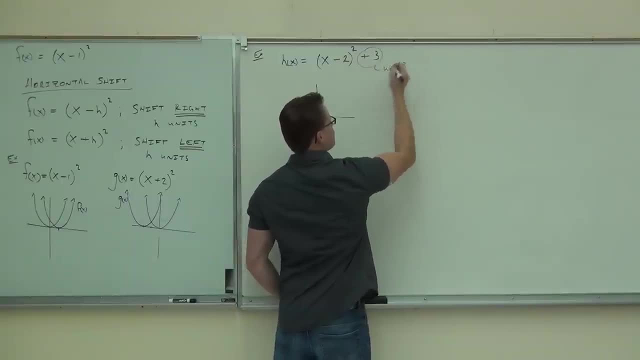 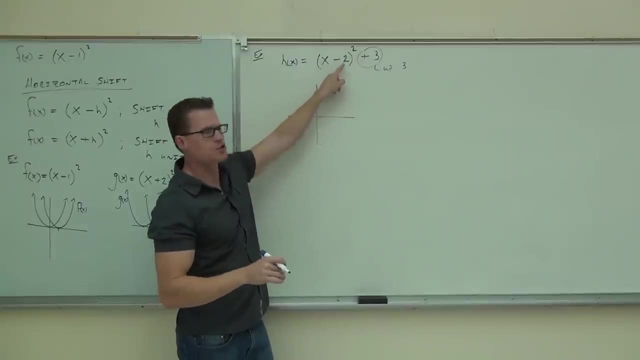 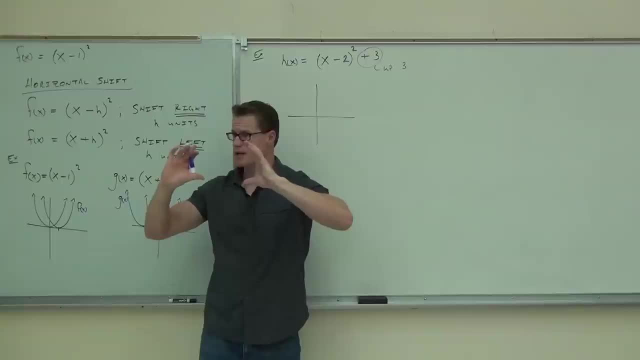 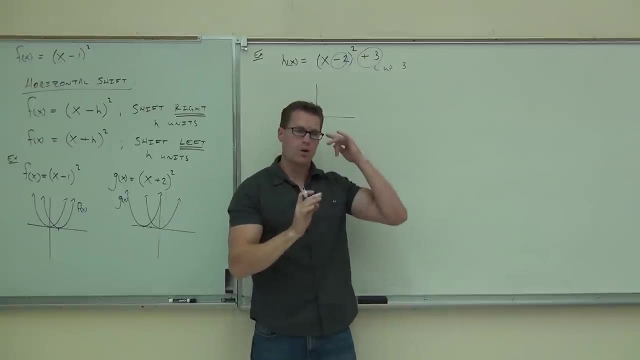 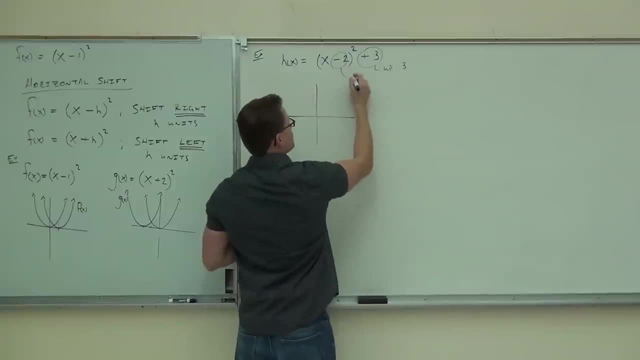 It's inside of our parentheses. there It was minus 2.. You can either think of it like well, I'm slowing it down, so start later, or you can think about that if it's inside the function it's kind of opposite of what you want to think. 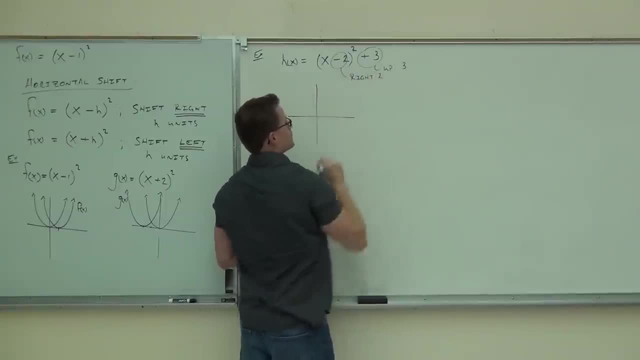 it is. This is going to be to the right 2 spots. So, from our origin, we're going to go up. You can draw your original graph if you want to. I'm not going to anymore, I'm just going to do this. 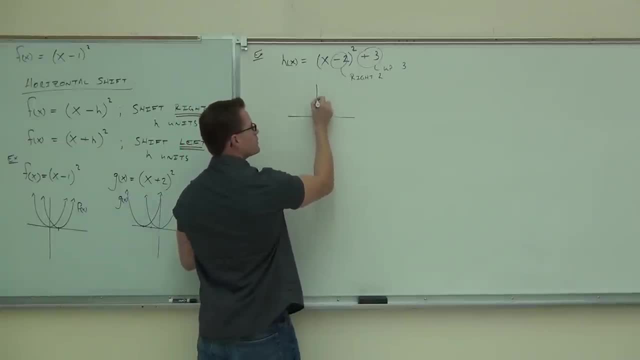 to graph it from the origin. we can go up three. we can go to the right two and we're going to put one little dot right there. Remember, you're not drawing lines right, You're not going up three, down two and drawing a line. 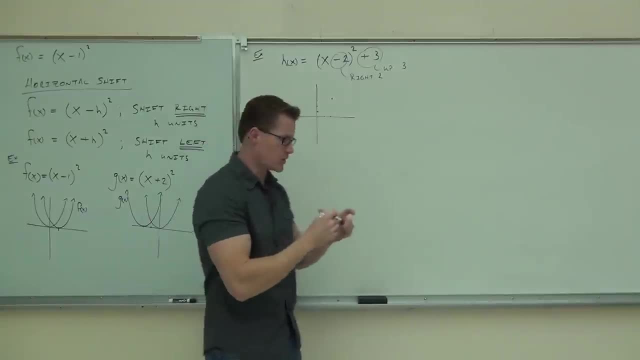 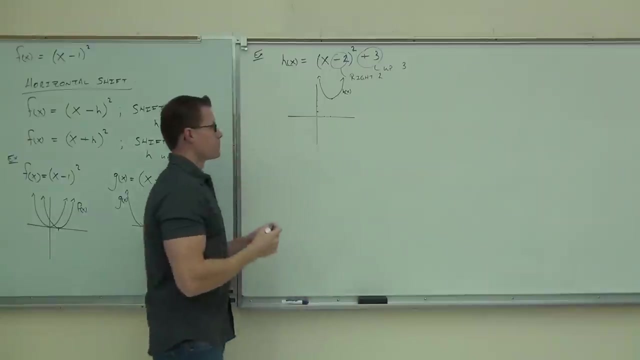 We're not talking about lines, We're talking about parabolas. We're graphing quadratic functions here. Then from there, after we go up three and right two, we'll redraw our original graph And label it. You guys still okay so far. 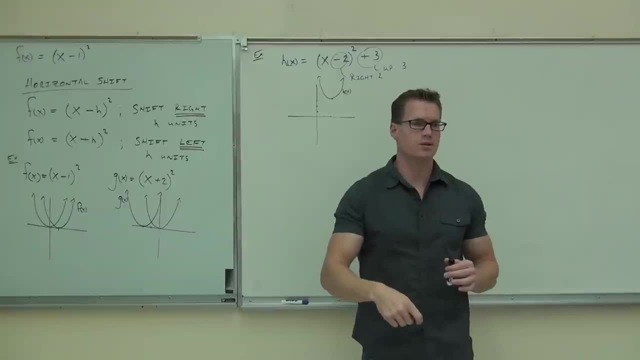 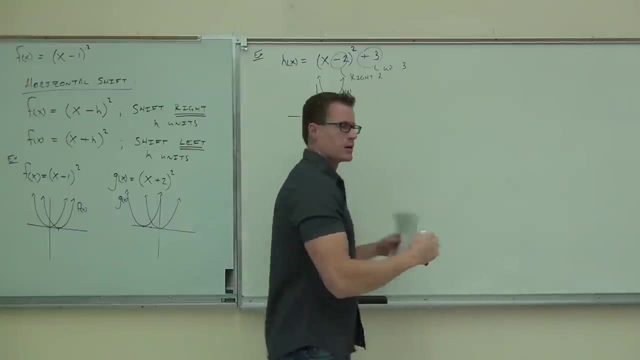 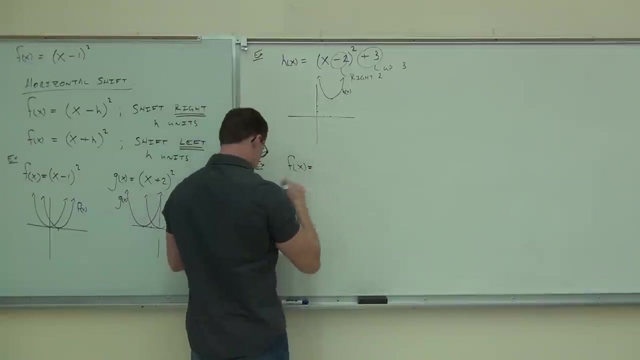 Kind of trudging through this pretty quickly, but it's a review of the old material, right, So it's kind of a nice refresher for you. hopefully Are you ready to try one on your own? Can you do that? Okay, let's do this one. 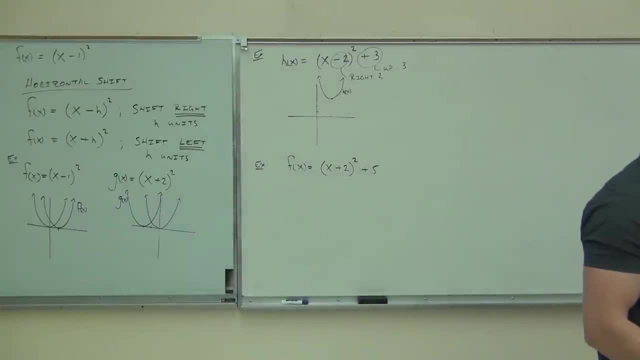 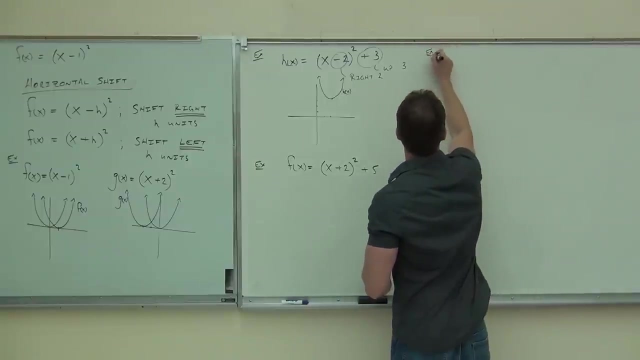 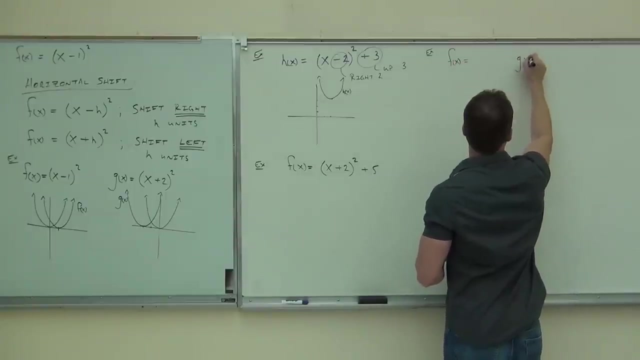 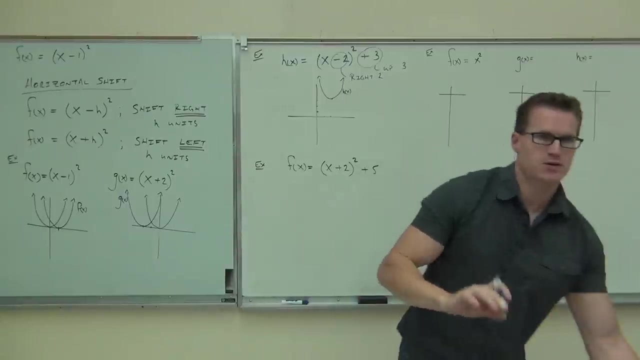 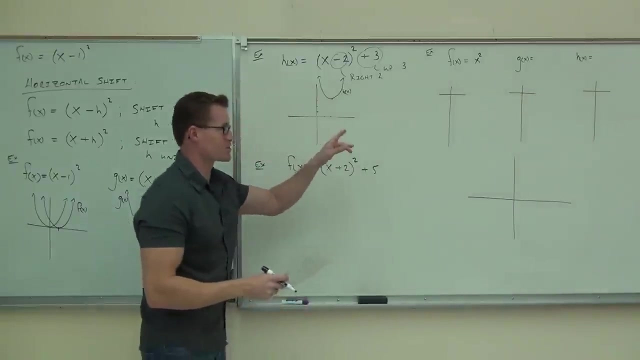 Here we go. I'm not drawing crosses here or anything. Those are tables. okay, I'm not doing that, But we're going to make some tables in just a second. By the way, I don't want you graphing these with tables. 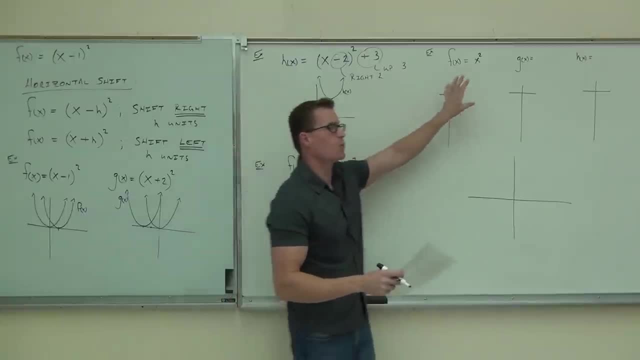 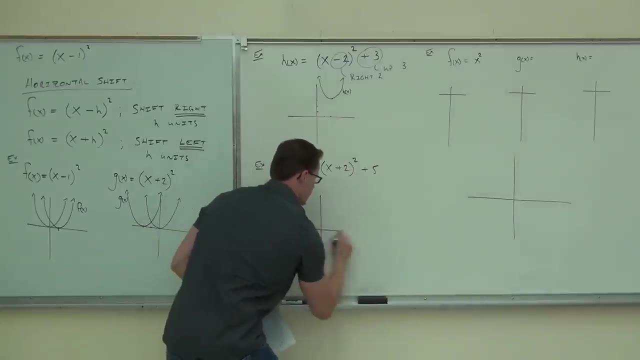 I want you graphing these with the shifting that we're talking about. I'm just going to show you one more thing. This is the only thing that you haven't seen before. We're going to talk about it over here Now. as far as this graph goes, of course we're going to read this from the right to the left: 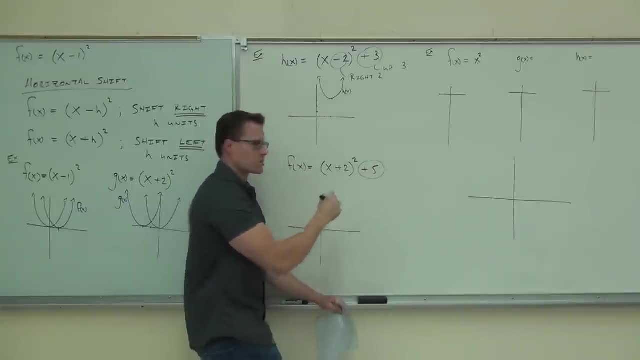 So this plus 5, everybody. what did the plus 5 do for you? Up 5.. Great, all right. So up 5,, no problem. How would this plus 2 inside of my function? what does that do? 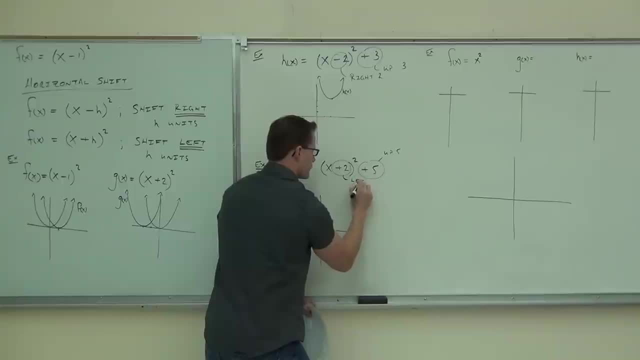 Left 2.. Left 2, great, all right, I like it. So we're going to go up 5, 1, 2, 3, 4, 5, up to the left 2.. We'll put our point right there. 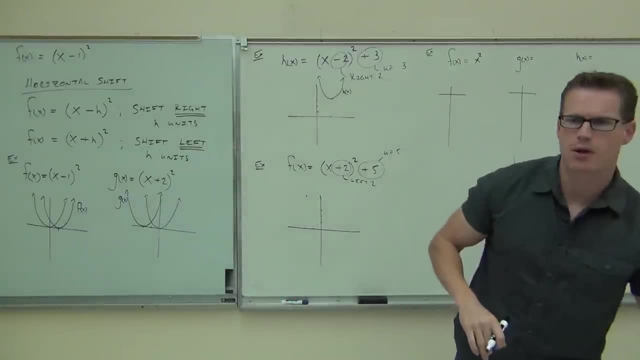 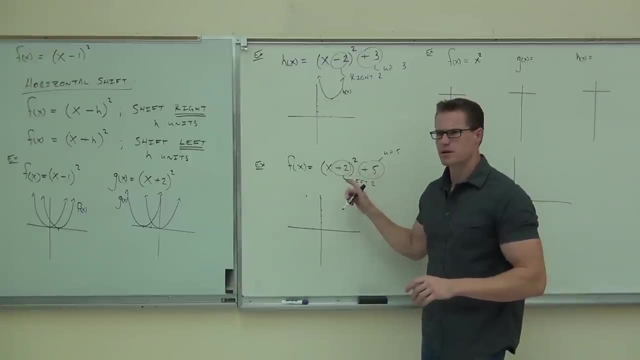 Let me refresh your memory on this. Is this going to be an upward-facing or downward-facing parabola, and why Upward-facing? because it's positive. What's positive, The 2,, the 5,, what's positive Before the x. 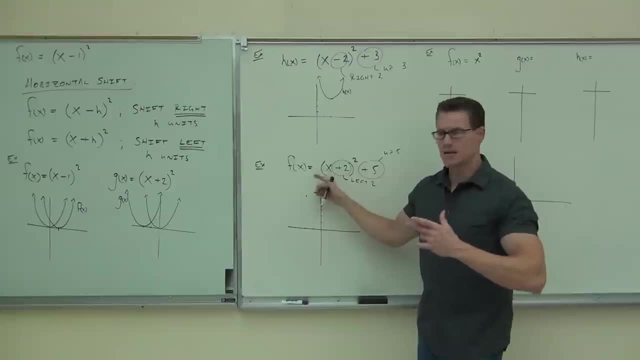 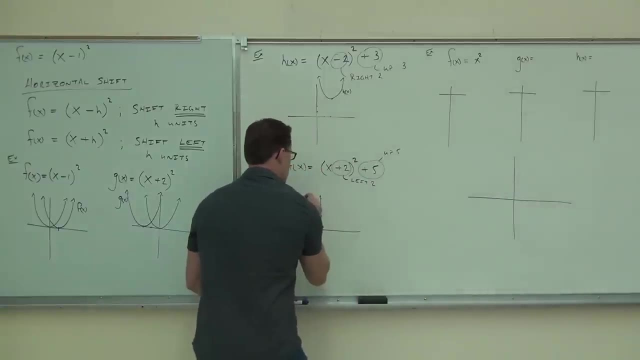 Ah, we look right there, don't we? If that was a minus or a negative, we would have this inverted right. We'd have it reflected. If it's not, it's going to be upward-facing. So this right here is still going to be upward-facing. 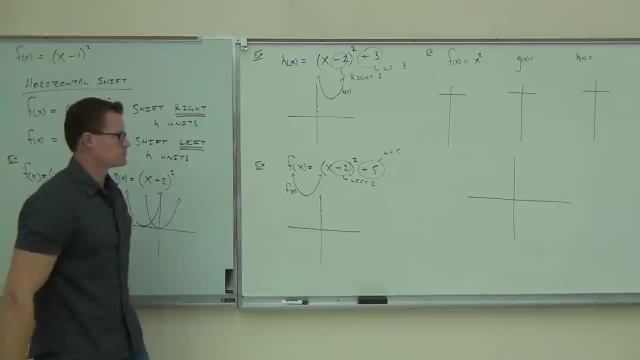 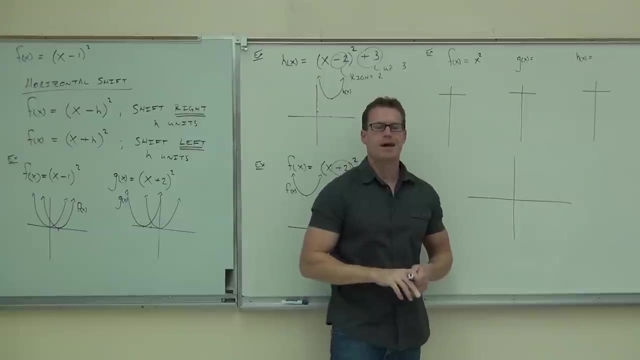 Make sure we label that f of x. and we got it Okay on a show of hands. how many of you feel okay with what we just talked about so far today? Good deal, all right Now. the only other thing that I need to tell you that you haven't covered yet is what happens. 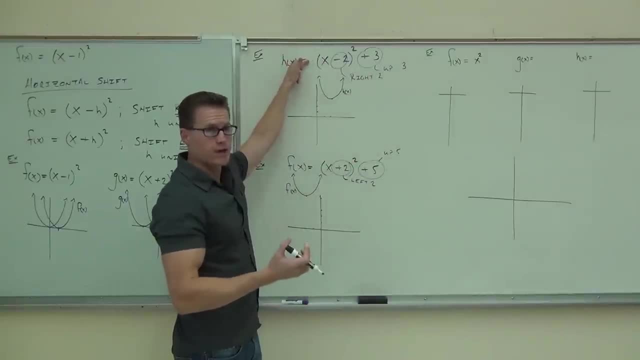 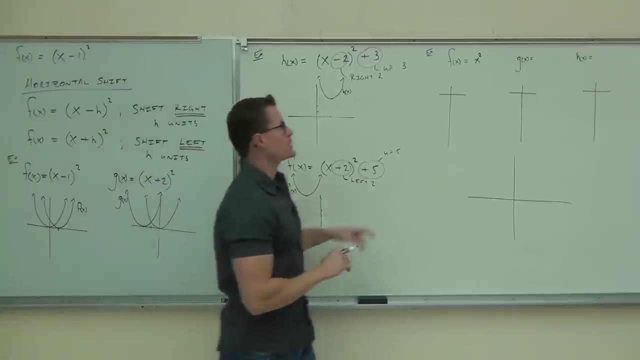 if there's a number in front of that besides 1? Because right now all you've seen in this class is positive or negative, but then there's been no number there. We're going to look at what a number does. So first we're going to compare x squared and see what that does graphically. 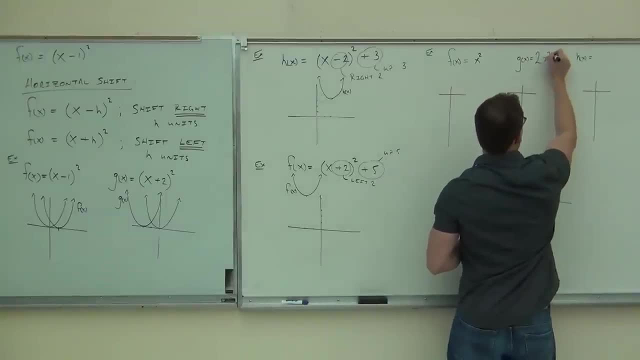 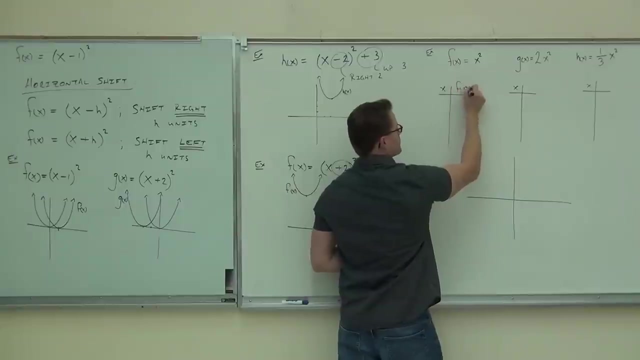 We'll compare 2x squared. and how about let's do 1 third and see what those things do? Now, of course, our tables are all going to have x over here, and they're going to have f of x and g of x and h of x. 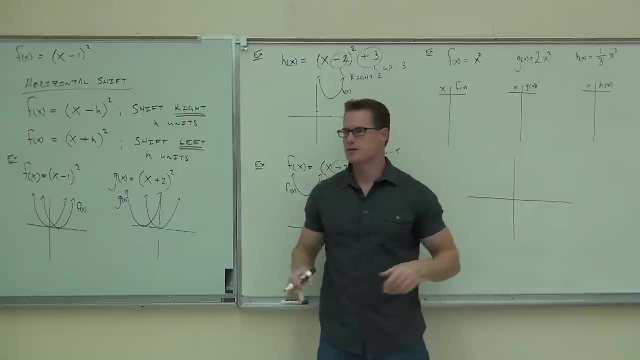 That just means what you're plugging in and what you're getting out. That's all that that does for you. So we're going to pick some points. We'll pick five points. We'll use the same exact five points in every case. 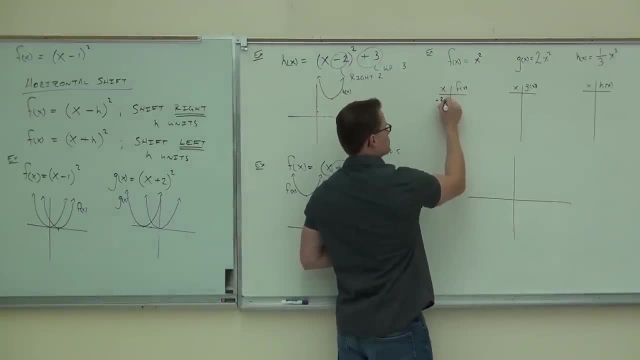 So we'll use negative 2, negative 1,, 0, 1, and 2.. Remember that when we're graphing things with tables which you don't have to do, you're going to be shifting, But when you're graphing with tables, you want to see what happens on the left. 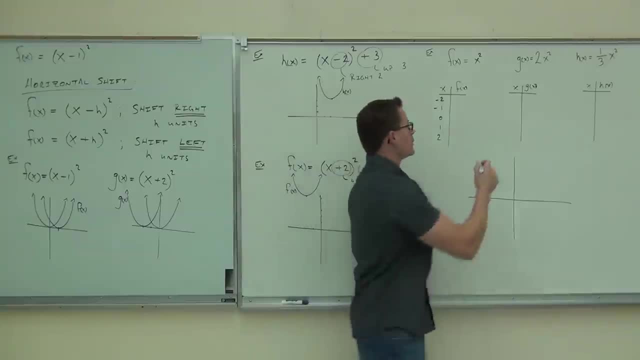 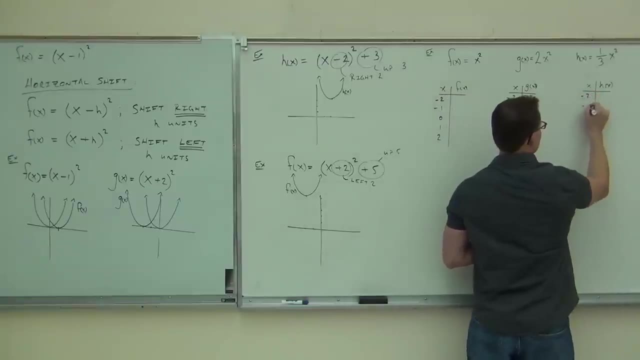 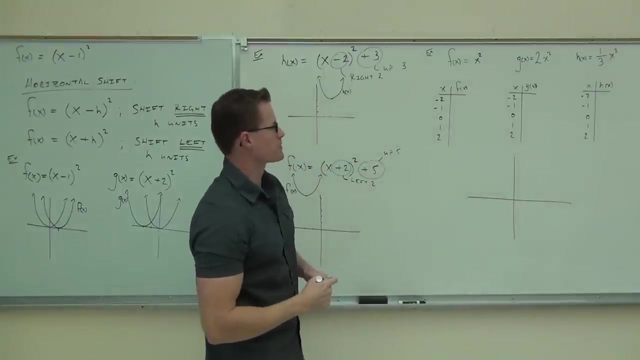 and the right side of the y-axis. so, positive and negative, We'll do the same thing here And here. Well, let's see about this. If I'm graphing x squared, this says you're taking these numbers and you're squaring them. 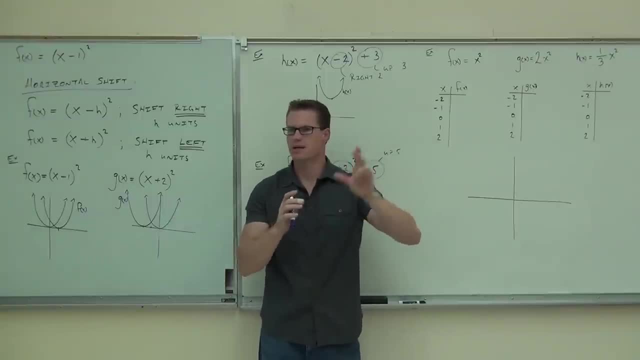 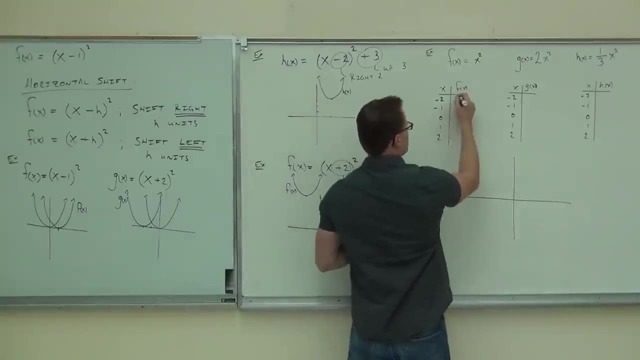 So can you help me out with that? If I plug in negative 2, how much am I getting out? Positive 4. Positive 4.. Why positive, not negative? Because, Okay, So this would be positive 4.. And then the next one would be: how much? 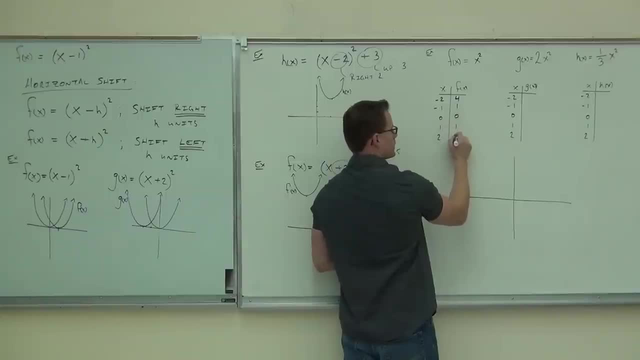 One, One And then zero, And then one And then four. Do you guys see my five points? I'm getting out of that, Yes, Okay, good, Now I'm going to graph that right now, just so we have that basic idea in our head and how. 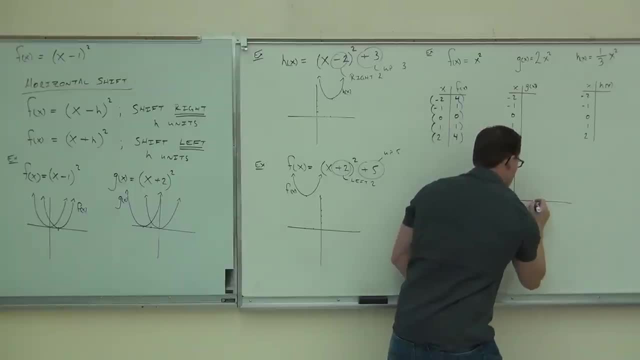 in fact we're actually getting these things anyway. So 0, 0,, no problem. 1, 1, 2, 4, negative 1, 1, negative 2, 4.. And sure enough, we get that nice basic graph shape. 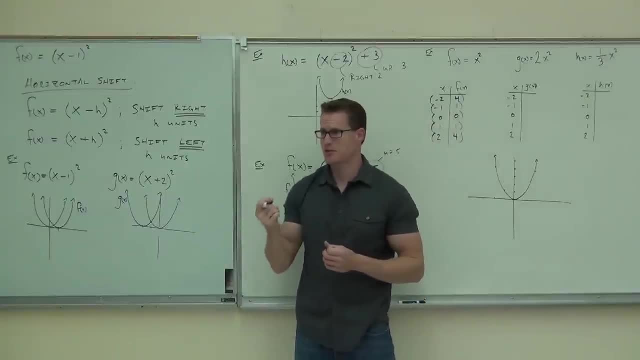 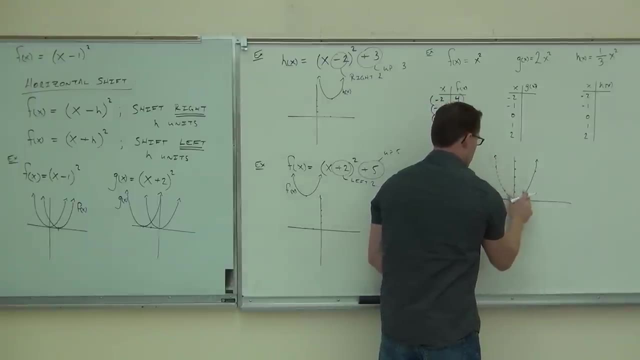 And I'm going to make this the dotted line because, well, I only have two colors and I have three graphs I'm going to draw. So the dotted line is going to be our original. So that's our F of X. So far, so good. 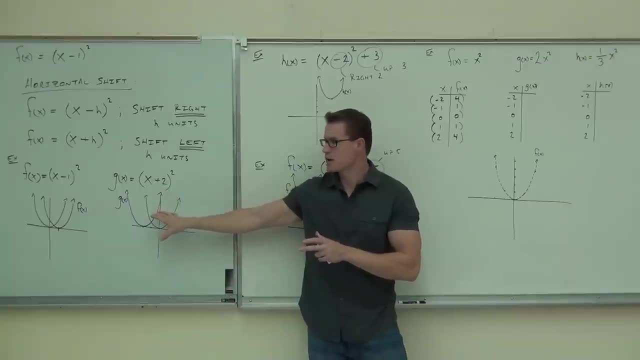 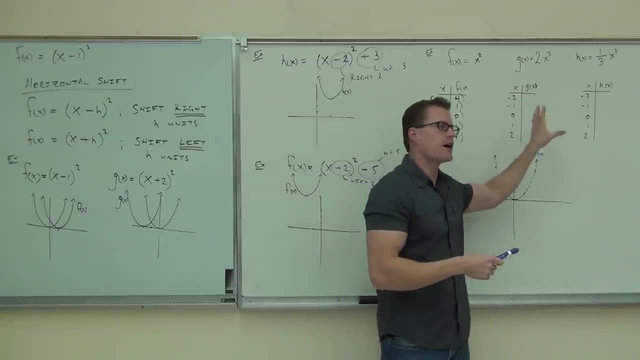 That's how our basic graph shape looks. That's why we got these things in the first place. That is our parabola. We just graphed those points, those five points. Now let's see what happens when we have a 2 or a 1 third in front of that X squared. 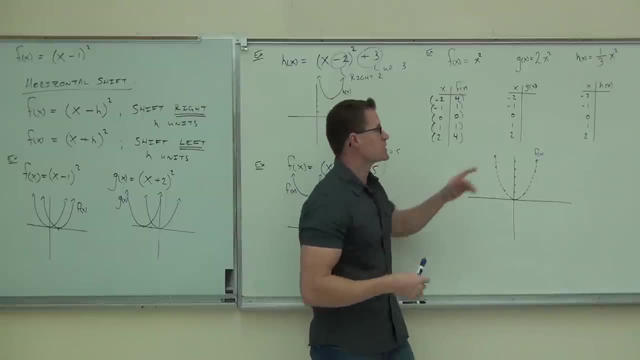 Notice what's happening. Please notice what's happening When you're with your operations here. this says you're going to square it before you multiply by 2. Are you with me on that? So let's go ahead and let's do this. 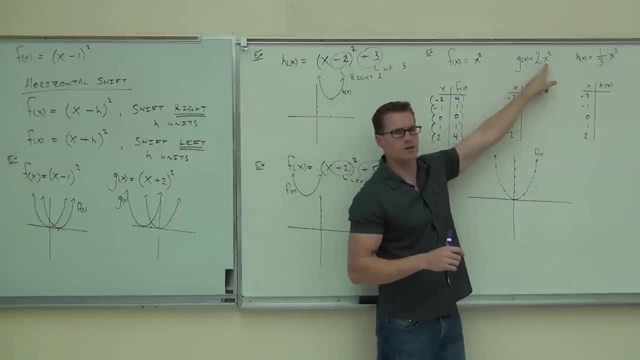 Let's do this together. Take your negative 2.. What's your negative? 2 squared 4.. Well, look, that's exactly what you've got here, right? But then you're multiplying it by 2.. What's that going to do? 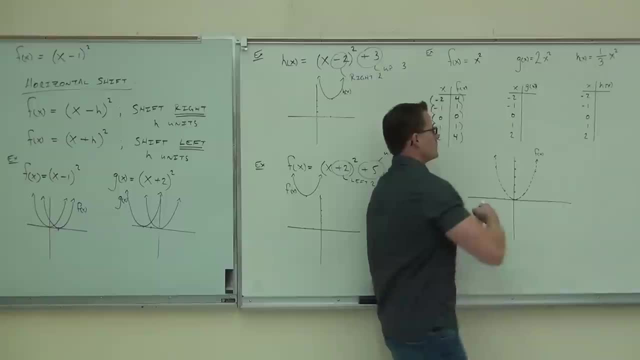 8.. It's going to really raise it up, isn't it? That's an 8.. Okay, Okay, So let's do the negative. What's negative? 1 squared 1.. And then you're multiplying it by 2.. 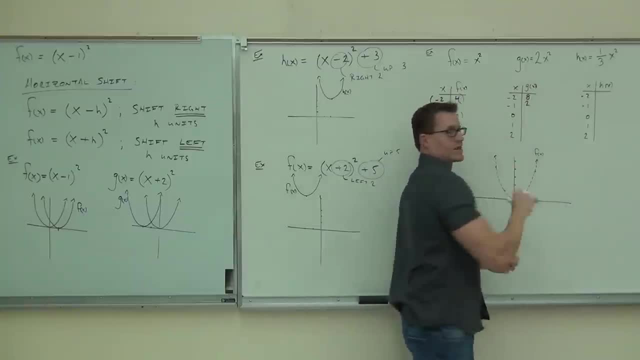 How much are you going to get Zero? I'll take care of the zero for you. Zero Zero is going to be 1.. It's going to be 0.. That's not going to change because even when you multiply 0. 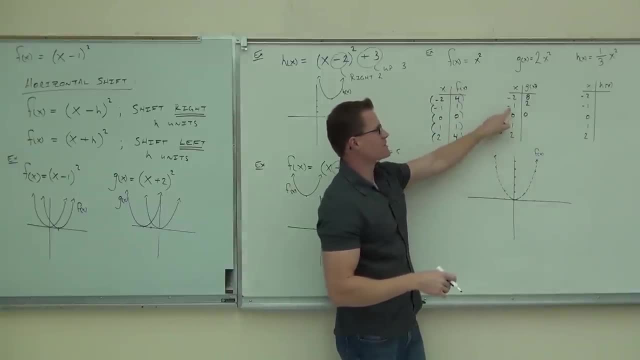 by 2, you still get 0.. 1 is going to be the same thing as this negative 1, because when we square something, we automatically get a positive out of it. So you're still going to get a 2 and an 8.. 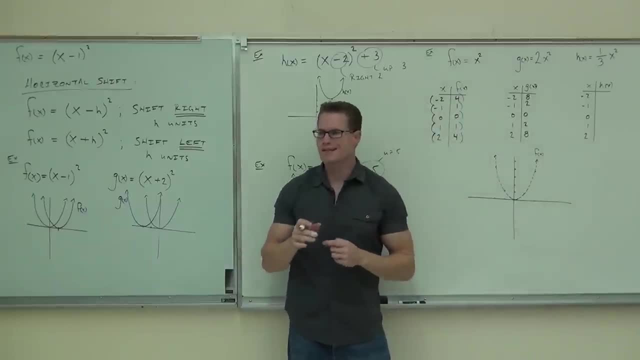 Are you okay with those points, ladies and gentlemen? So what did this essentially do to your graph? What did it do? It made it a narrow. It made it. what now? Skinnier Made it skinnier. Why, Well, look at it. 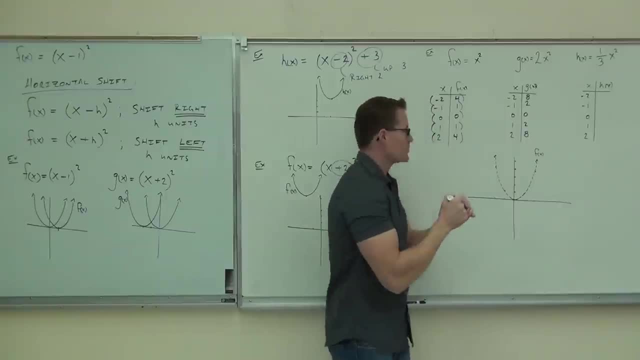 If you had it, just lost some weight. right, This is, isn't that weird. You multiply by 2 and you lose some weight there. It's getting thinner because what's happening? for every point you're making it climb a little bit faster. 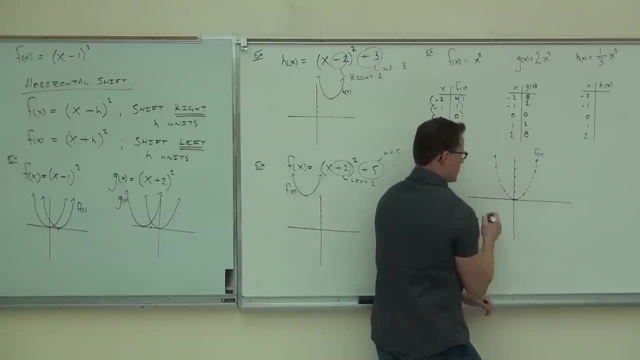 So you still have the 0, 0.. Yes, But instead of negative 1, 1,, you have negative 1, 2.. That's here, And instead of 1, 1, you have 1, 2.. 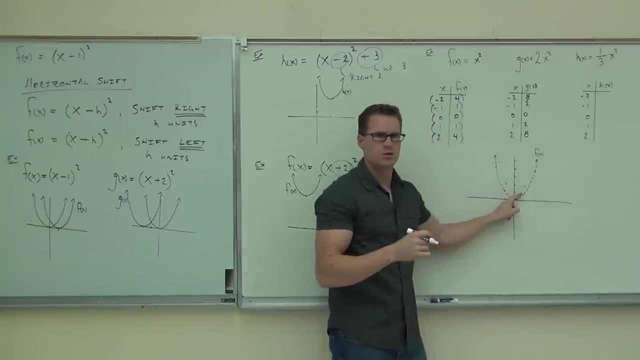 That's here. So move this point up by a factor of 2.. It said, oh, I'm going to double your height. That's what it did. I'm going to double your height. That's what it did. I'm going to double that height. 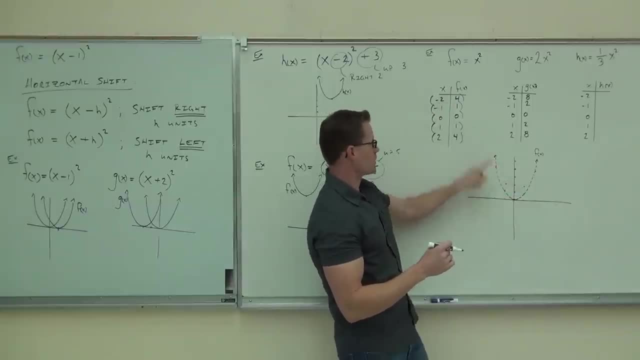 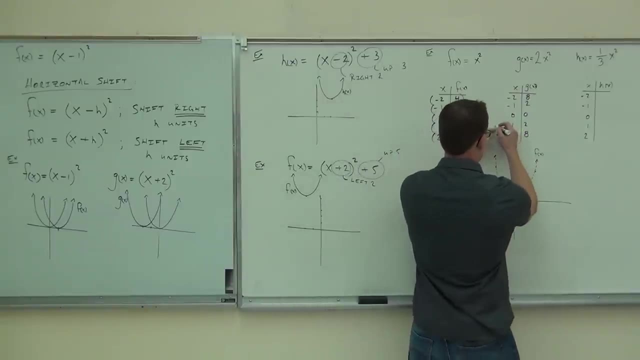 Now the next one: at 2, at negative 2, we were at 4.. Here we're at 8. That's doubling that height. That's way up here. Negative 2, 8. That's like here. 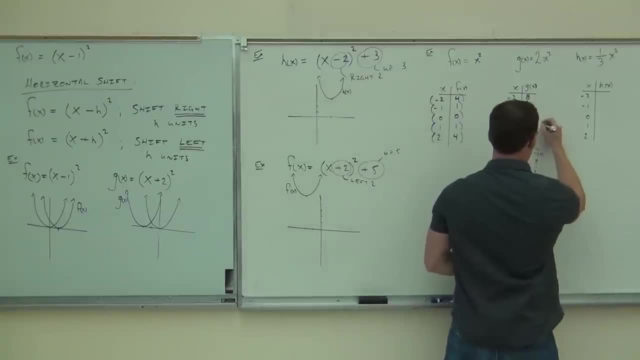 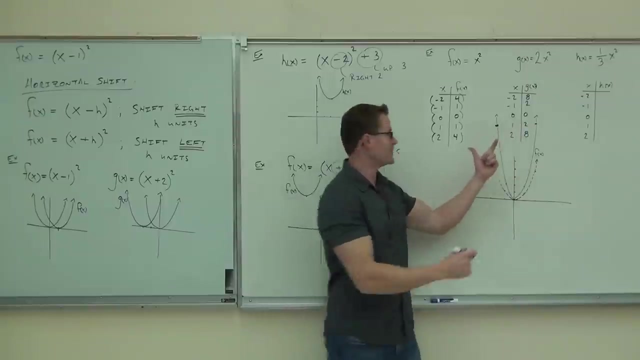 And positive 2, 8.. That's like here, So this graph is much more narrow. Can you guys see the graph? Okay, I'm going around that table. Actually it kind of looks kind of cool. And this is G of X. Still, so far, so good. 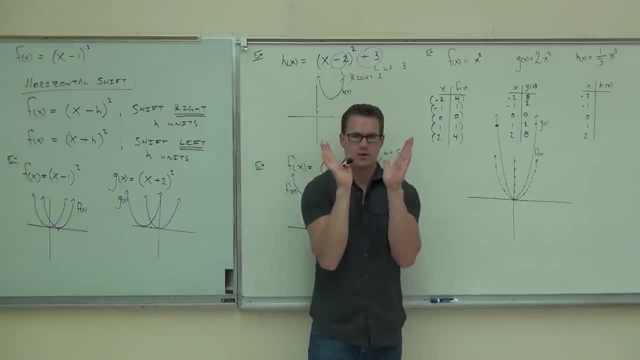 So when we did that, we actually shrunk it. Well, not shrunk it, but we squeezed that graph, Because it's taking every point, multiplying it by a factor of 2, that's doubling the height, That's squeezing it together. 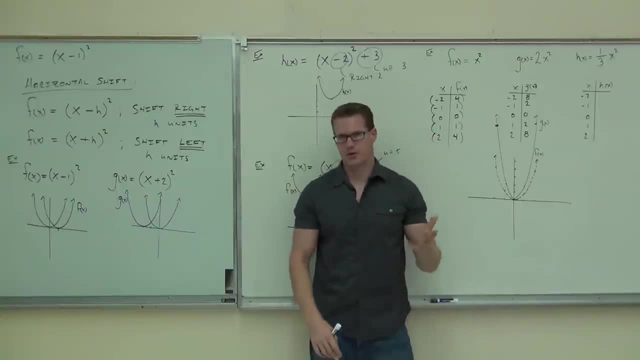 It's saying you're climbing faster. What do you think the one-third is going to do? Make it bigger. What do you mean? bigger, Wider, Wider, Wider. Why, Well, let's see, Let's do this together. 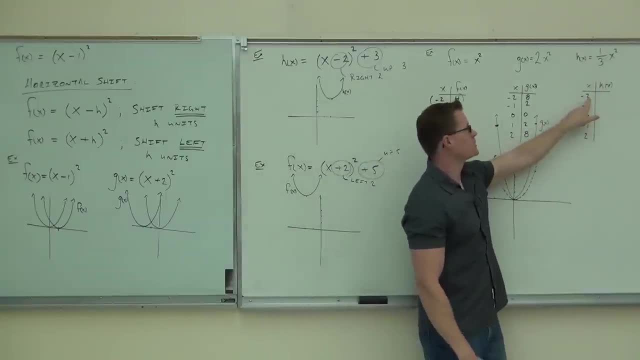 Remember, the one-third comes after you square it. So take your negative 2, square it. What's the square of negative 2,, please, 4.. And then you multiply it by one-third. So basically you cut it in thirds. 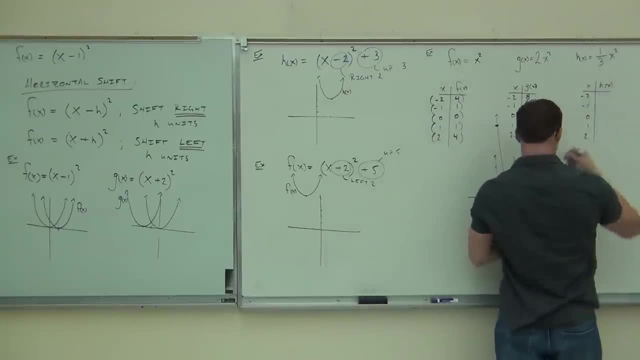 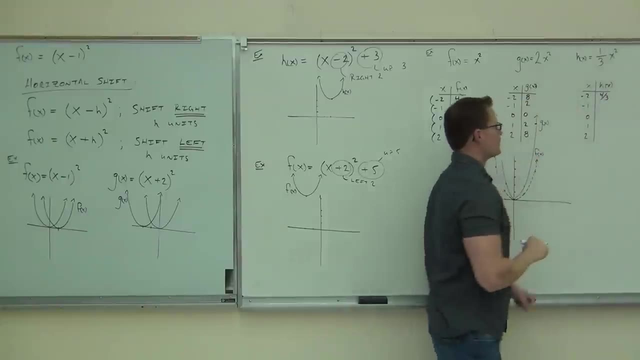 That's going to be four-thirds. Four-thirds or one and a third. Let's do the negative 3.. What's the negative 1?? If I square negative 1, I get 1.. But when I multiply by one-third, I get one-third. 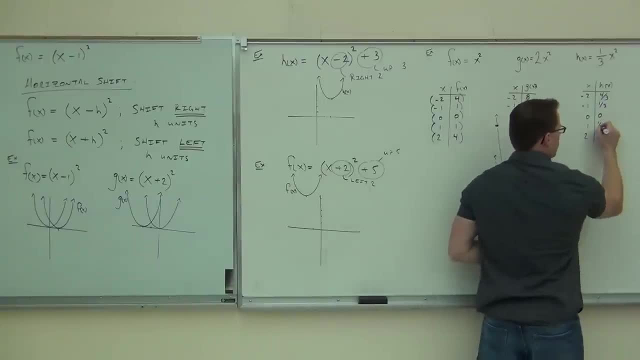 Zero, Nice, Zero One. again, you're going to get one-third, Because when you square a number before you multiply by one-third, it's going to be positive no matter what. And here we're going to get four-thirds. 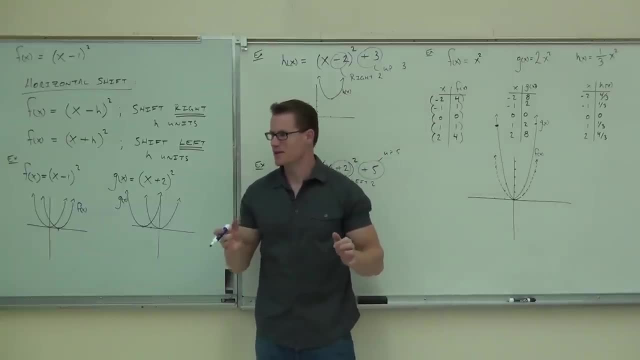 Now we've got fractions. Don't freak out on the fractions. I know it's only Wednesday. It's not Fraction Friday, all right, But don't freak out, We can do this. We took a fraction. We do still have our five points, only this time. 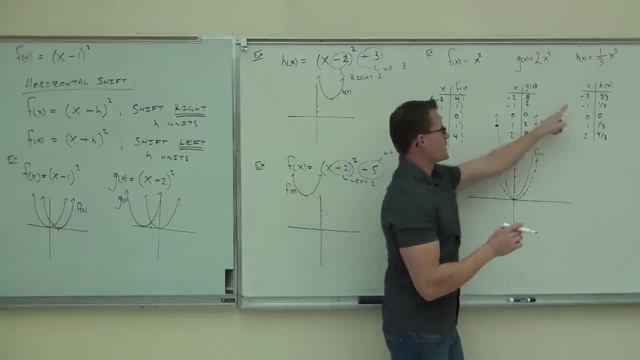 instead of being negative 2, 4, that's here- we're negative 2, four-thirds. We've cut it in thirds. Four-thirds is one and a third. So negative 2, one and a third. That's right here. 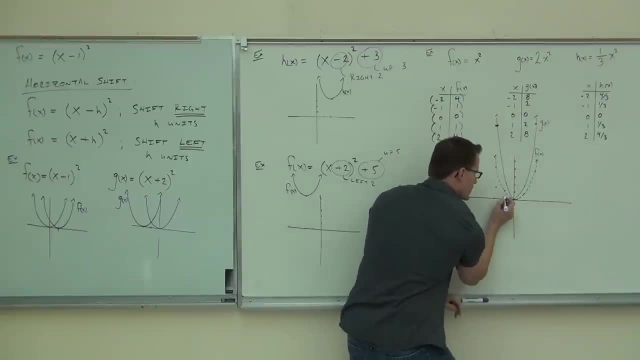 Then we have negative 1, one-third. That's like that's right here. Do you see how it's going to widen out right there? It's going to widen that side. Zero, zero, no problem. One one-third, two four-thirds. 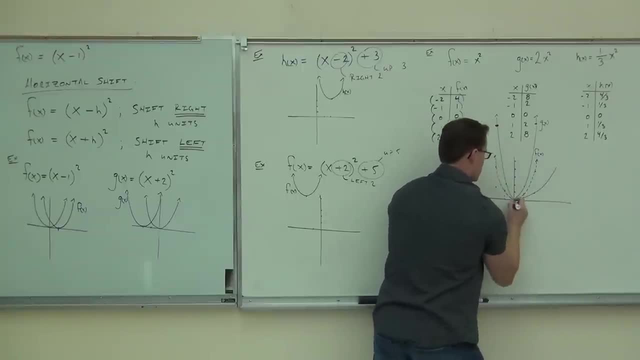 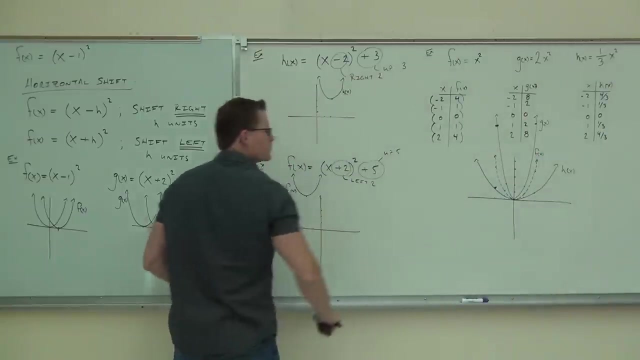 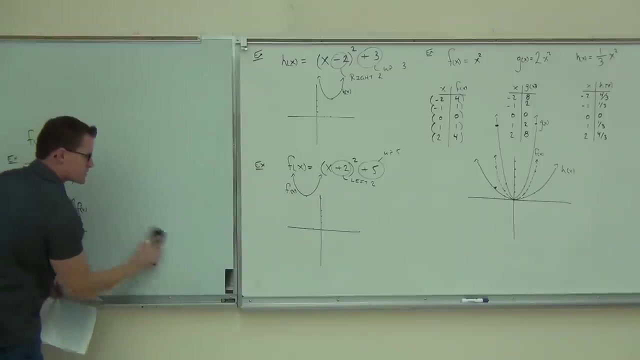 That's one and a third. And we did this graph, So those numbers in front of those parentheses are going to be negative: 2, one-third, two, four-thirds, That's one and a third. They're going to mean something for us now. 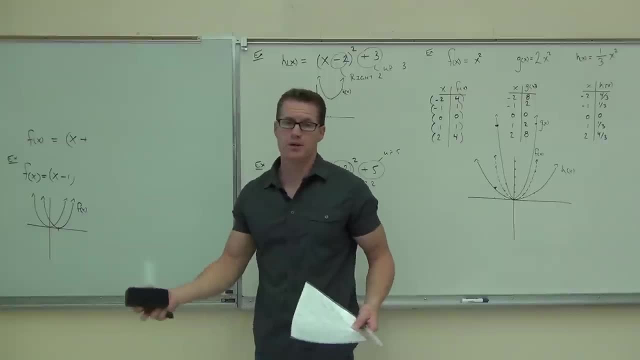 They're going to tell us what our graph is going to look like, even more accurately than what we could do before. It's going to tell us whether we have a skinnier graph or a wider graph. Now we are still curve sketching. 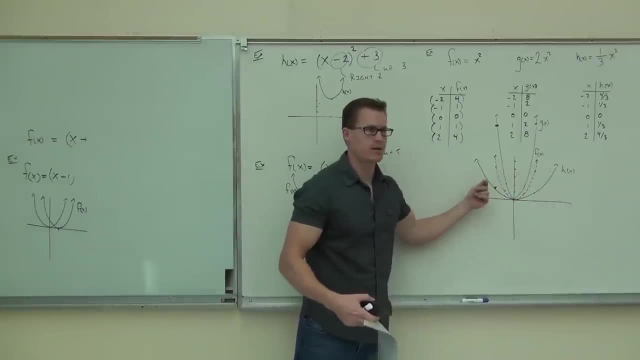 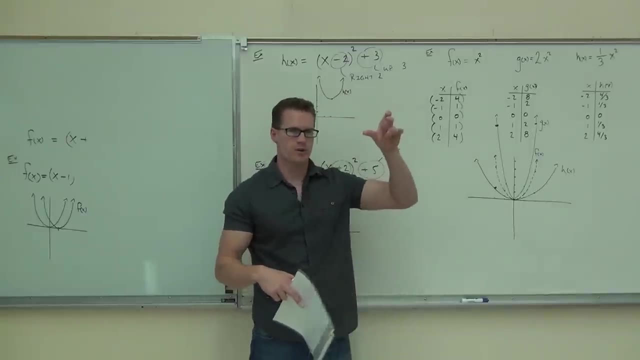 We're not going to be exact on this thing. These are pretty close to exact and we did that with a table. We're not going to be using tables, So pretty much here's what I want you to do. I want you to look at the number in front of the parentheses. 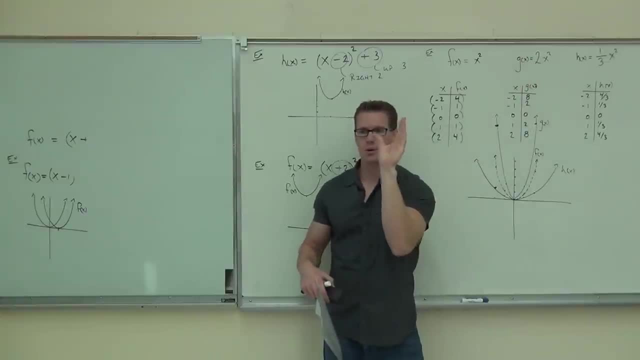 If it's a 2, a 3,, a 4,, you're going to make your graph narrower, narrower, narrower. Does that make sense? If it's a fraction that is less than less than 1,. less than 1, you're going to make it wider. 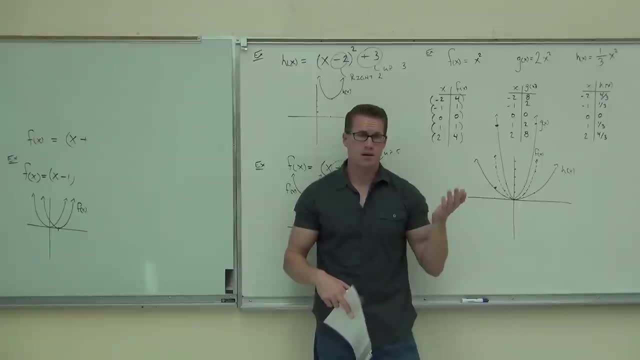 Why do I say less than 1?? Because it's one of the ones still going to make it wider. If I give you like 5 halves, if I give you like 5 halves here, 5 halves is 2 and a half right. 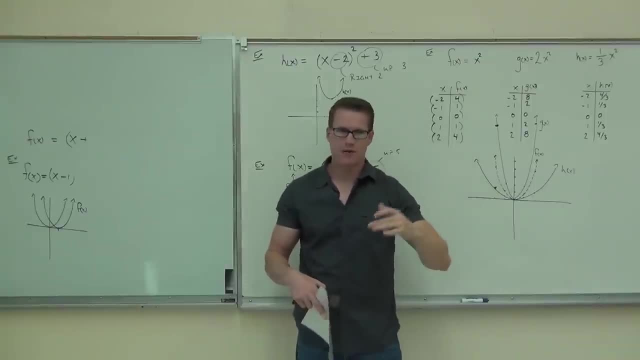 So don't just look at the fraction, Look at the value of the fraction. Fractions don't automatically mean wider, but if it's a fraction less than 1, like one-third or two-thirds or something, yes, it's a little bit wider. 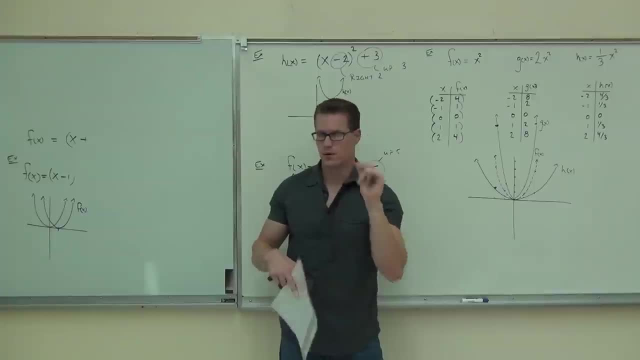 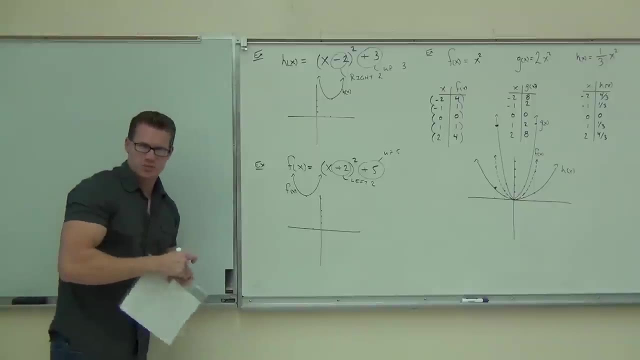 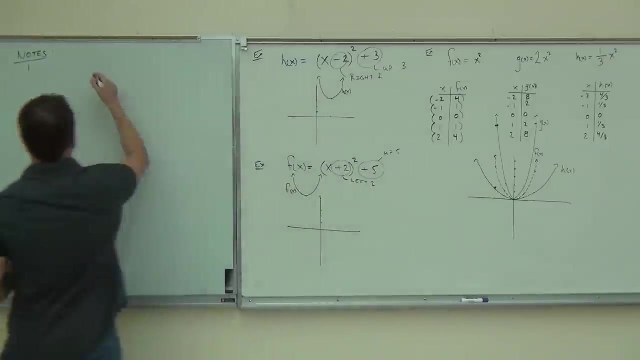 Does that make sense to you? Yes, no, No, Okay. So a couple of notes for you. Okay, So a couple of notes for you. The value of a in that ax squared bx plus c is pretty important for us. First note, if that value of a is positive. so, for instance: 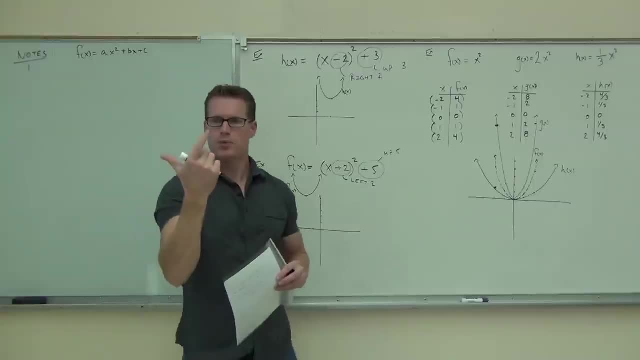 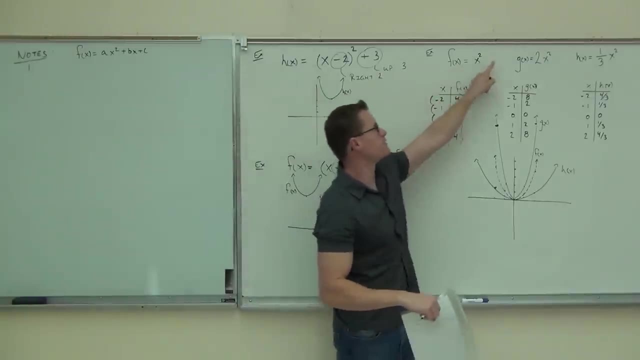 if that a is positive, is our graph going to open up? It's going to open upwards or downwards Up. It's going to open upwards all the time. That's when this is positive, and that's positive, and that's positive. 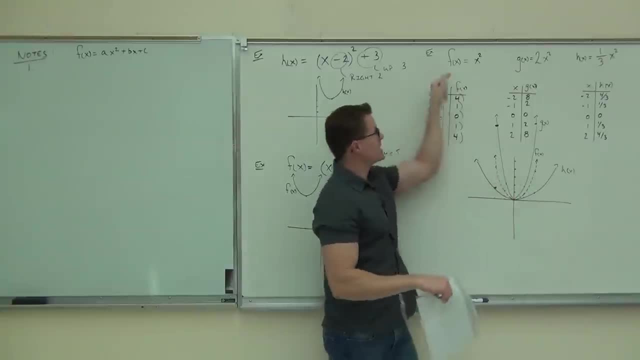 Look at all those graphs open upwards. Are you with me on that? If it's negative, negative, negative, negative, it's going to change all these numbers to negative, which is going to take every one of those and flip it upside down. 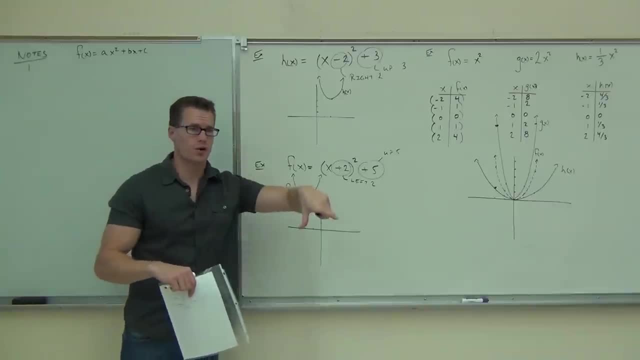 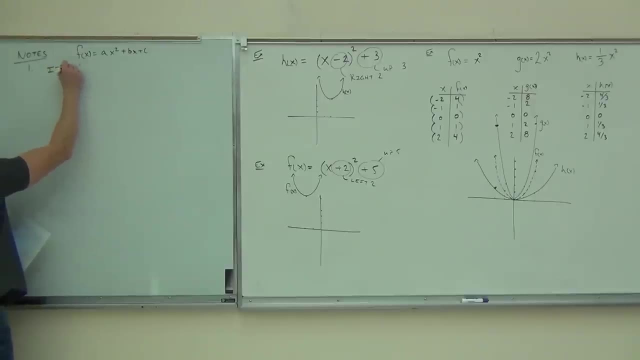 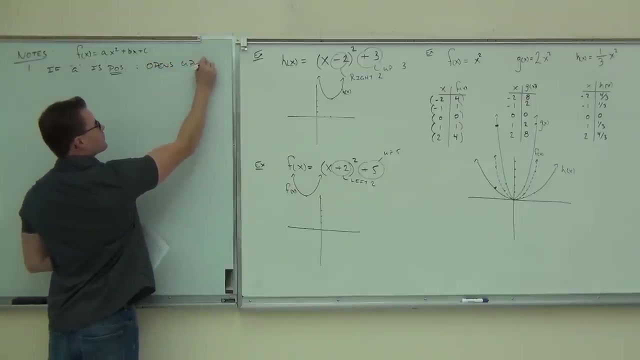 So if a is positive, upward opening. If a is negative, downward opening. If a is positive, it opens upward Or faces upward or has a smiley face because it's feeling up. It's positive. Get it Smiley. 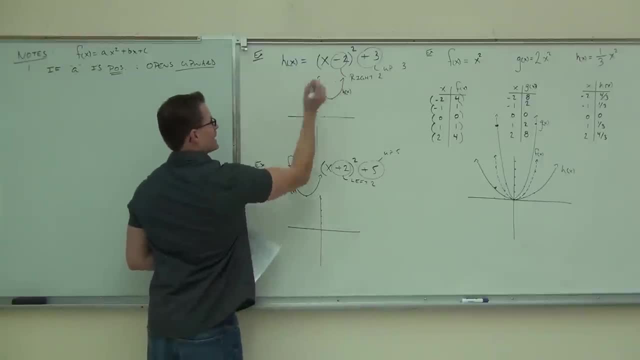 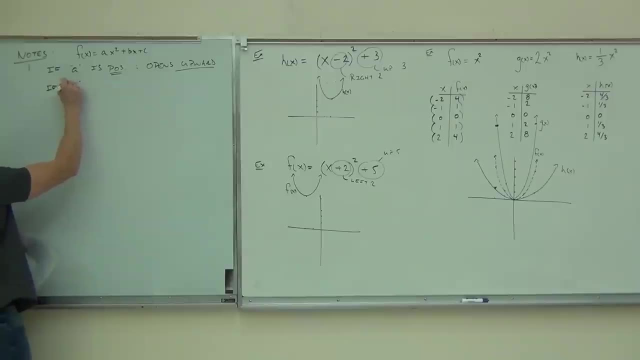 Those aren't points. I just made a smiley face. Okay, So if a is positive, it opens upward. If a is negative, it's feeling down, It's frowning downward, like that. So if a is negative, it's opening downward. 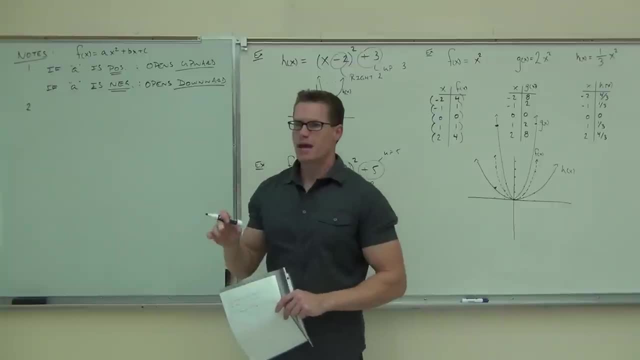 A is positive, opens up, A is negative opens down. If a is greater than 1, are you going to have a narrower graph or a wider graph? If a is greater than this, is our a right there. Notice how that's our a. 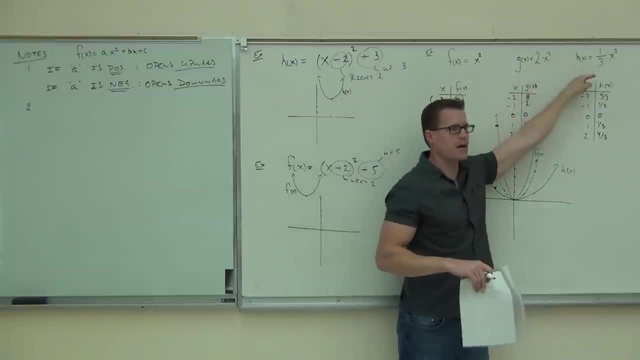 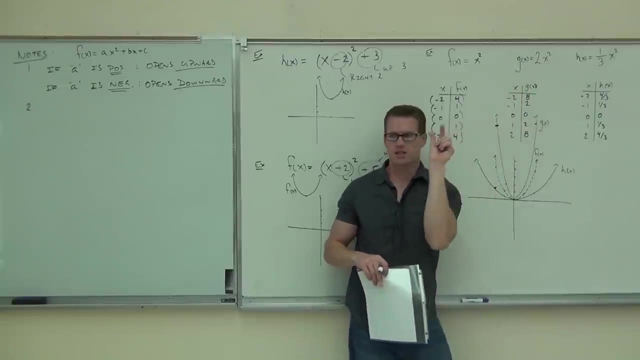 That's the number in front of x squared right. So, even though I have nothing else after that, that is still my a. You follow: If a is greater than 1, we're going to have a skinnier graph or narrower graph. 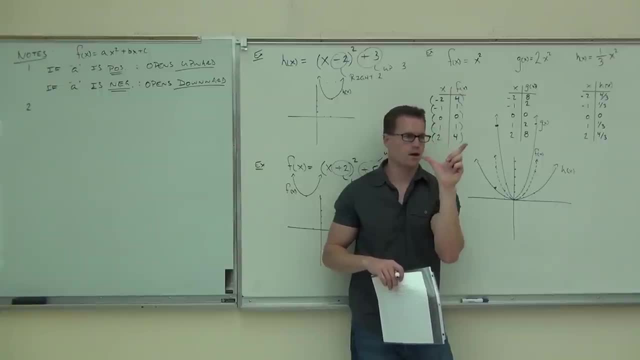 If a is less than 1, we're going to have a wider graph. That's less than 1.. That's 1. 3rd, We're going to have a wider graph. You with me. Now I'm going to tack on one thing to that. 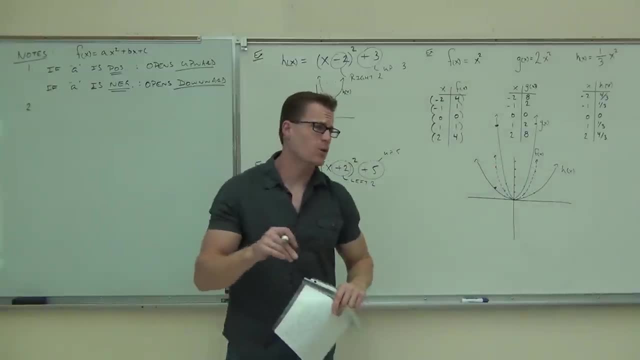 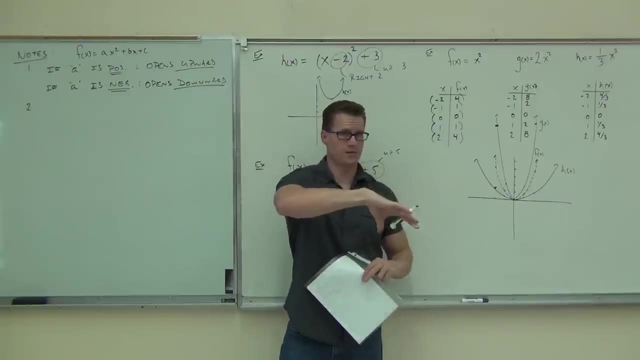 I'm going to say the absolute value of a, And the reason why is because I don't want you considering the negative when you're considering how wide or narrow the graph is. That negative simply tells you upward facing or downward facing if it's negative. 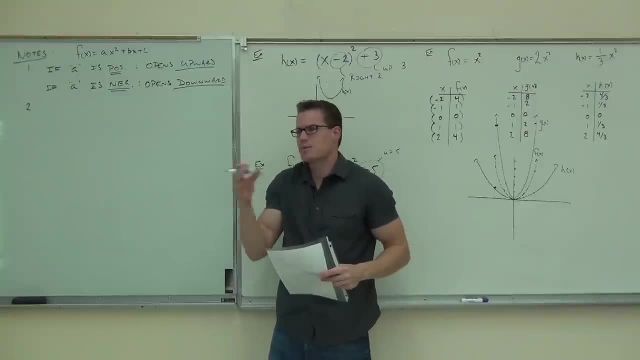 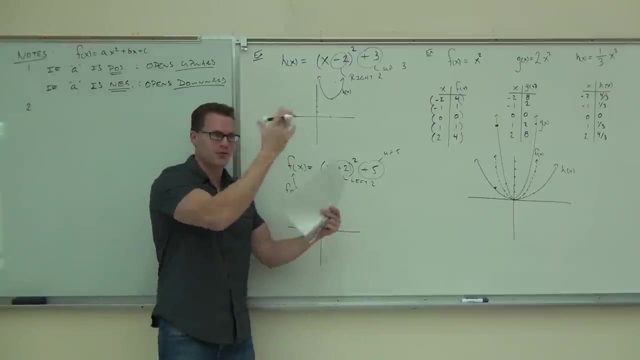 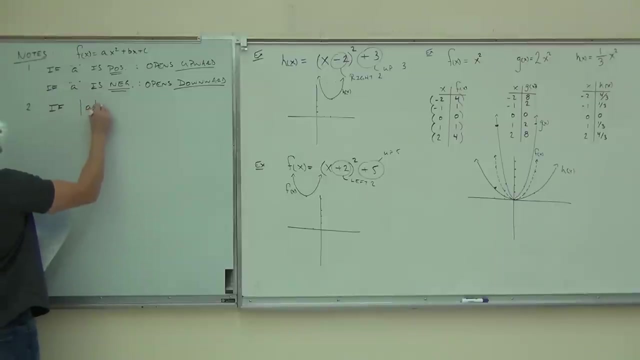 You follow. So we look just at the number value, So that the absolute value to tell whether you're narrow or you're wide. Well, not whether you are narrow or wide right, Whether you're graphed or not, If absolute value of a is greater than 1, so you're looking at that number in front of x squared. 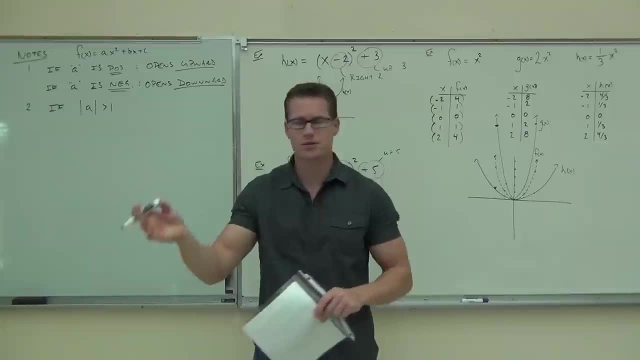 If it's bigger than 1, so even if it looks like a fraction- 5 1⁄2, 7 3rds 2. If that's bigger than 1, you're going to be narrower. The graph is narrower. 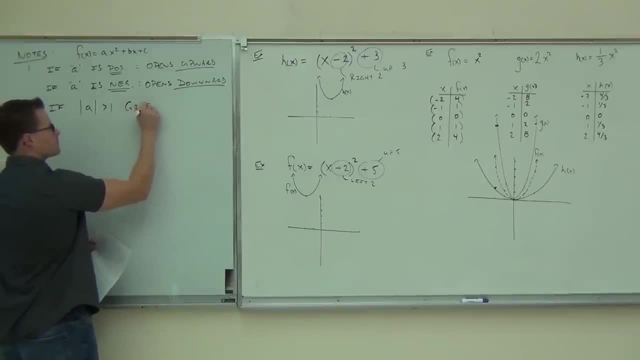 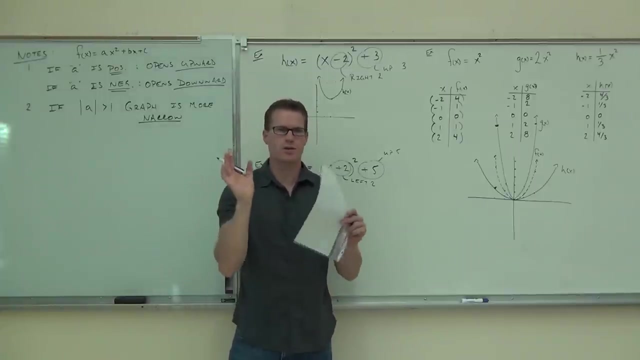 And the larger the number, the more narrow it is. So it's not just automatically: either you're one way, or you're narrow, or you're wide. okay, The bigger the number. If I had a 10 here, it would be increasing these numbers by a factor of 10.. 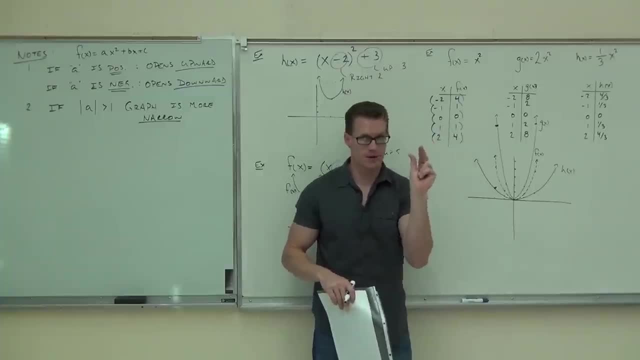 It would be very, very, very, very skinny. You follow me on that Very skinny. So the bigger the number, the more narrow we have If a, If a is- and we're talking, of course, absolute value- less than 1, so we have a fraction there. 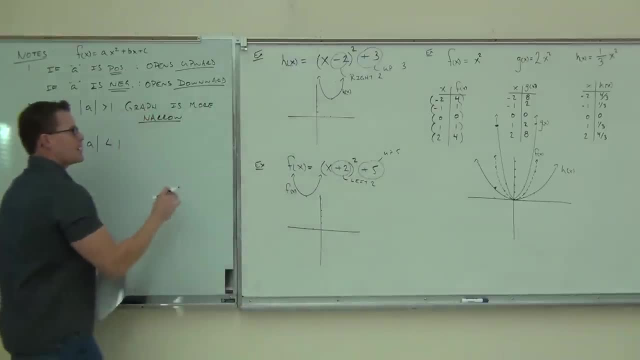 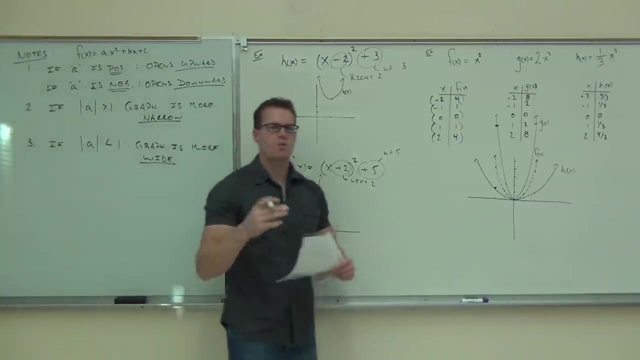 If it's less than 1, so between 0 and 1 in absolute value, we're going to have a more wide graph And of course, the smaller the number, the wider we get. If I had 1 10th here, oh my gosh, it would be very shallow. 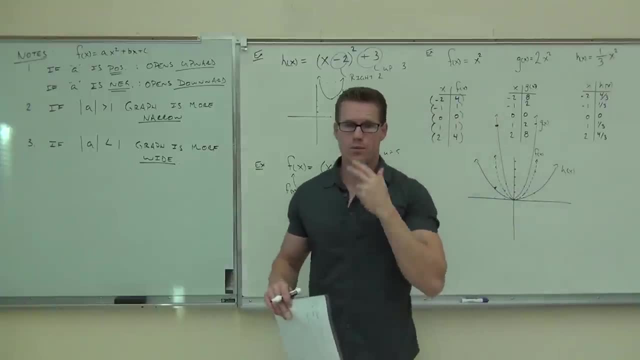 It would be going way out here Very shallow, Very shallow, Very, very wide. So when you're graphing these on your shifts, yes, you can go up or down, No problem, That's that You can go left or right. 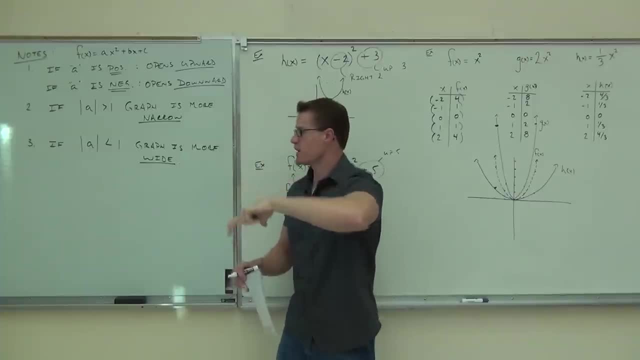 No problem. That's that You're now going to be able to tell whether you're upward facing or downward facing. That's because we know the positive and negative for our a. We've only done that. This is the new one, right here. 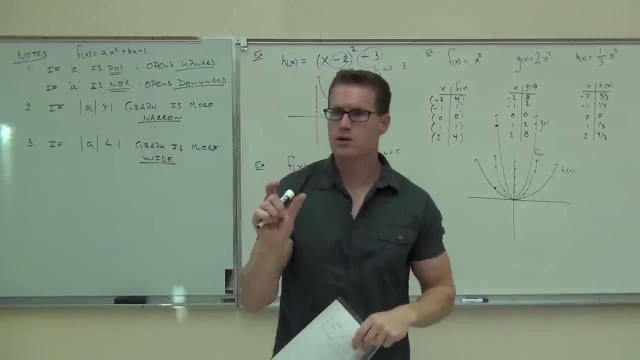 You're going to look at the number in front. If that is bigger than 1, you're going to make it more narrow. The larger the number, the more narrow you make it. So 3 is going to be more narrow than 2.. 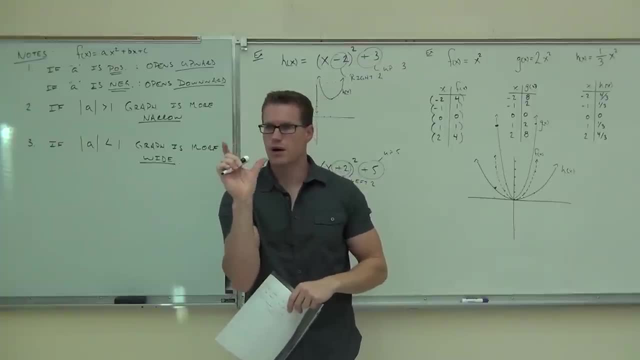 You follow me. Or 1. 3rd is going to be wider, 1 5th would be even wider, 1 10th would be even wider. So we're going to look at those numbers and draw our graph accordingly. 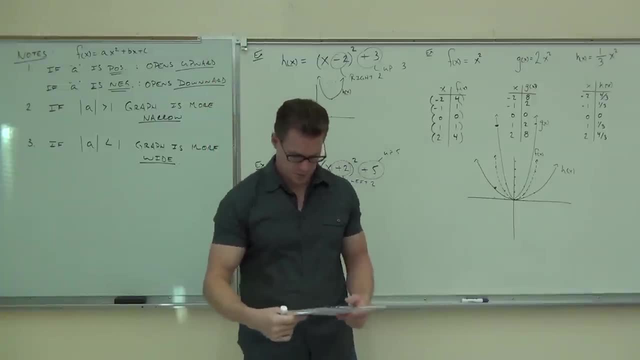 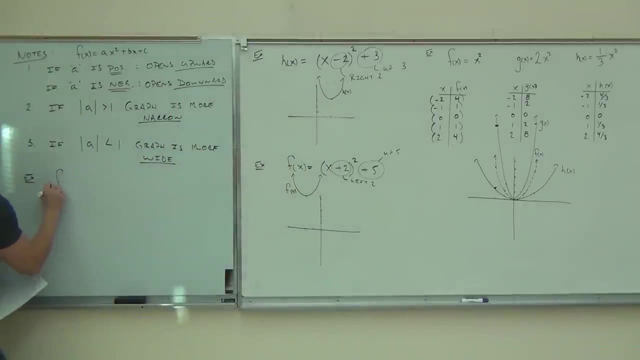 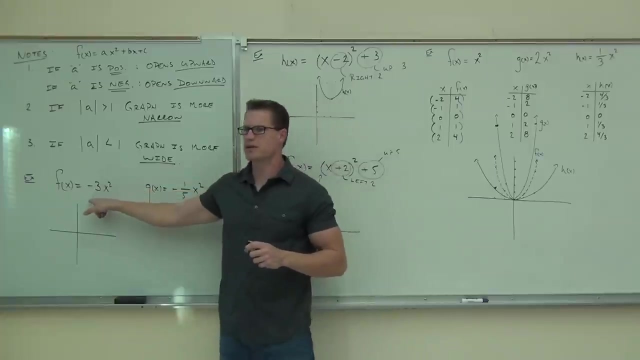 How many of you feel okay with what we've talked about so far? Good, Good. Let's try two very quick examples Here, Just basic ones. This one: This is negative 3x squared. Ladies and gentlemen, is it still starting at the origin? 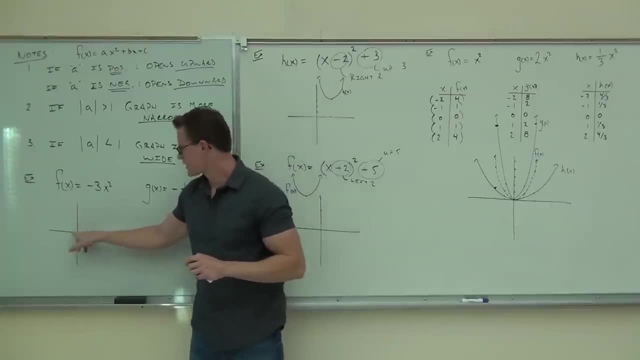 Have I shifted it up, down, left or right at all? No, So it's still starting at the origin. Is it going to be upward facing or downward facing, Downward facing, Great. Is it going to be wider or narrower? 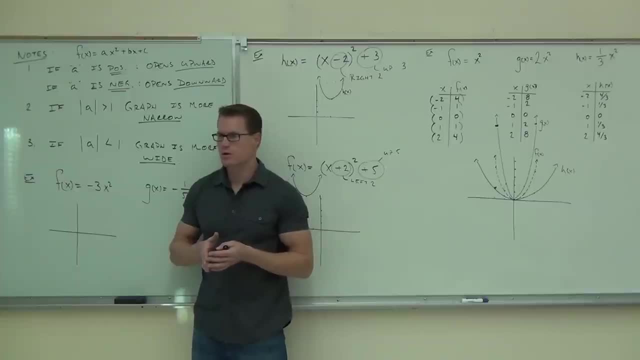 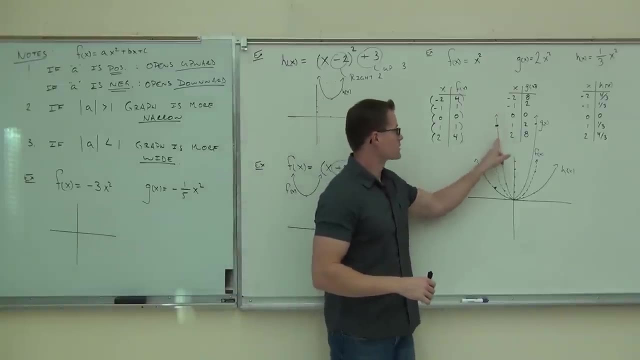 Narrow. Why narrower? Because it's greater. Okay, An absolute value. We ignore the negative. You look at the 3. That says narrower. Is it going to be narrower, Narrower or wider than this 2x squared? What do you think? 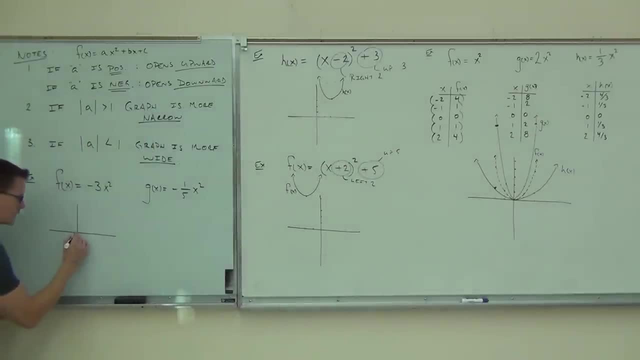 Narrower. That's a pretty narrow graph. This one's going to be downward facing, sure, but it's going to be pretty narrow, So don't just give me one. You don't have to be exact here. Okay, We're still sketching. 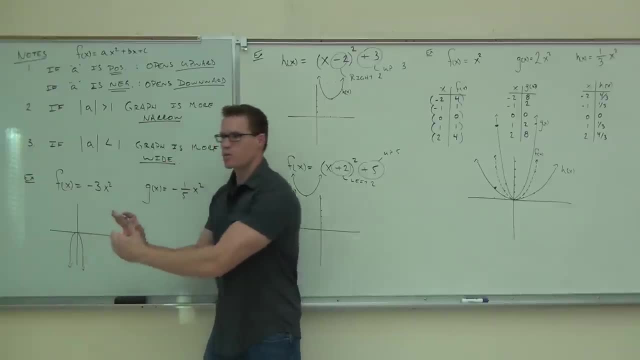 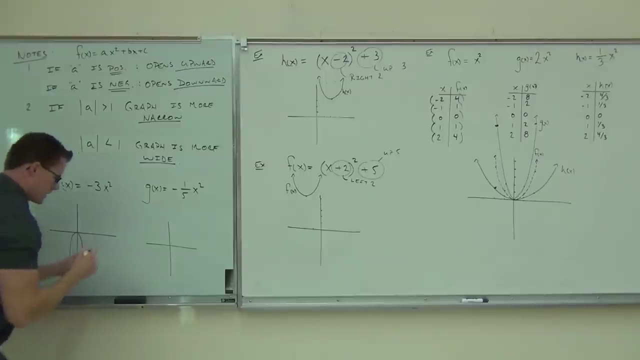 Don't just give me one type of parabola anymore. You need to determine whether it's a narrow parabola or a wide parabola. Of course, that's f of x. Now the next one, g of x. 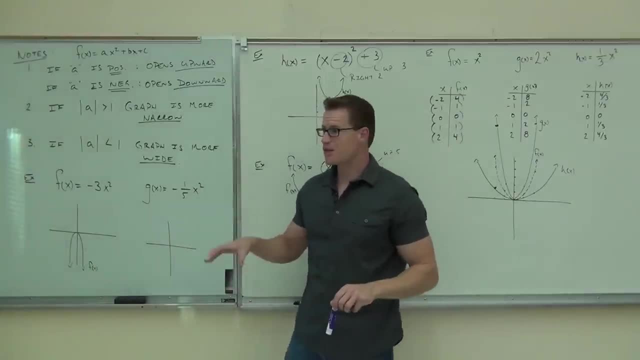 Is it upward facing or downward facing? Downward facing: Is it still at the origin? Yes, Sure. And is it wide or narrow? Wide, Wide, Pretty wide. How wide? Wider than 1.. Yeah, Pretty darn wide. 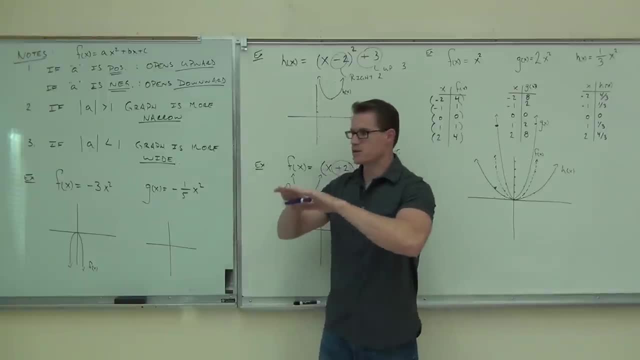 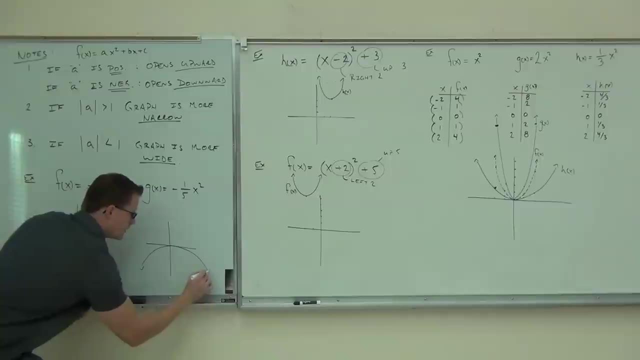 I mean, this is 1 third. That's wide already, So 1 fifth is going to be even flatter, even more shallow. So here we go. Okay, I want to represent that that's pretty wide. Now, of course we're not exact because we don't have those tables. 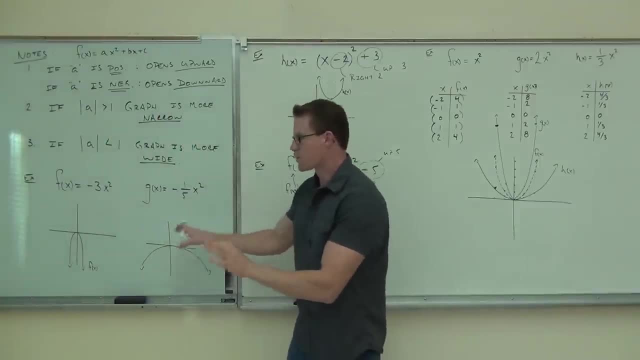 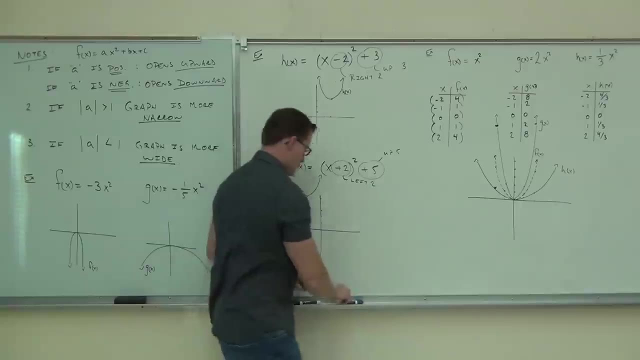 All right, We don't know exactly what that looks like, We have no other points, But we're going to estimate that that's about what that looks like. Hmm, So, in general, here's what we have going on with our quadratics. 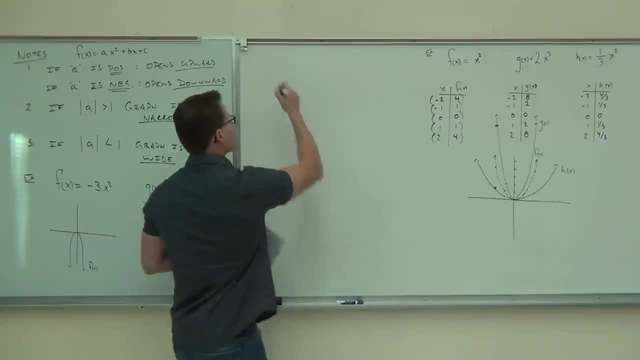 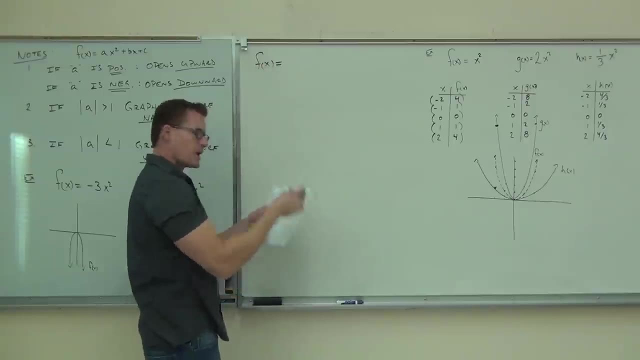 We're going to put all this stuff together. We're going to mine every single piece of this. So here's what all of your graphs in this section are going to look like. You're going to have some function name: f or g or h. 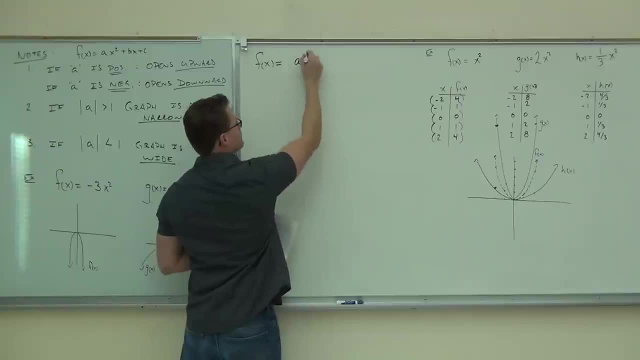 It doesn't really matter. You might have some number out front, You might have some parentheses. I'm putting a plus minus there. Now we're not doing quadratic equation or anything. okay, I'm saying, it could be a plus or a minus. 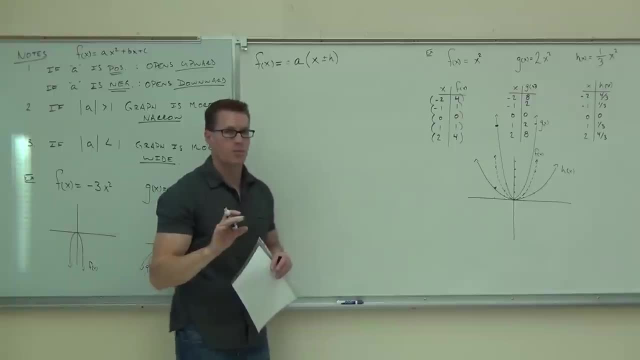 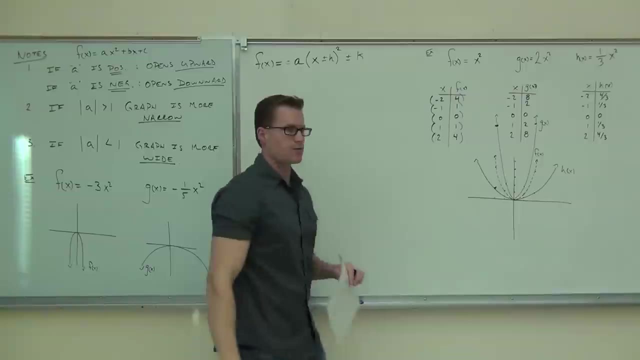 Out here. you could have a plus or a minus. The plus wouldn't show up, but the negative would. You'll definitely have a square, and then you could be adding or subtracting something at the end of your function. What you're going to do on every problem, and especially on the test. 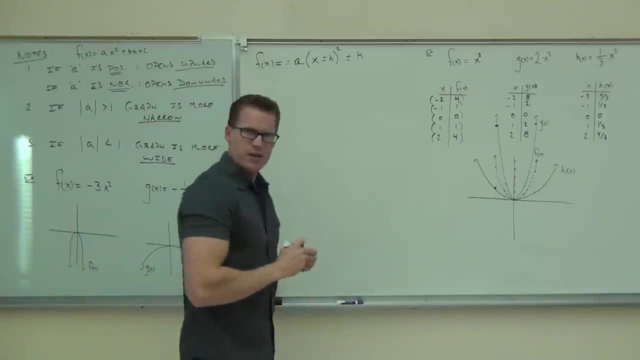 you're going to circle those parts and tell me what they do. Remember doing that from the chapter 8 stuff. We're going to do the same thing. You start at the right-hand side, This plus or minus k. that should tell you something. 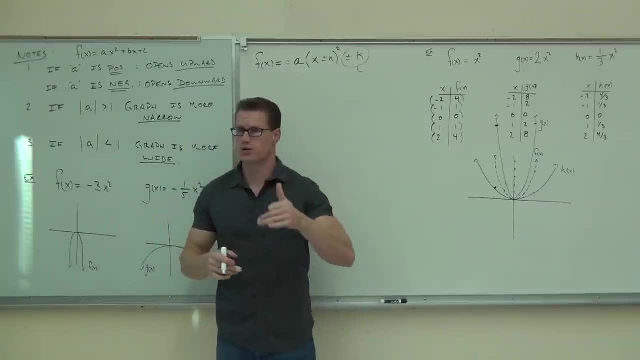 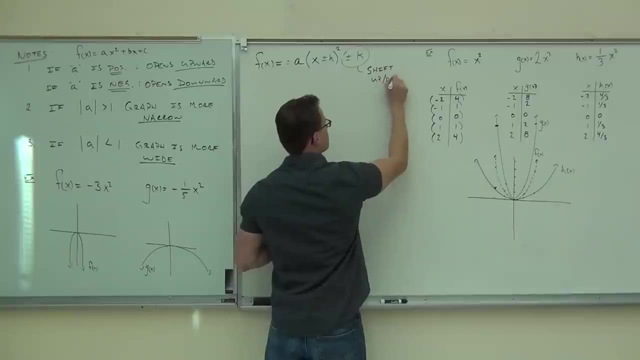 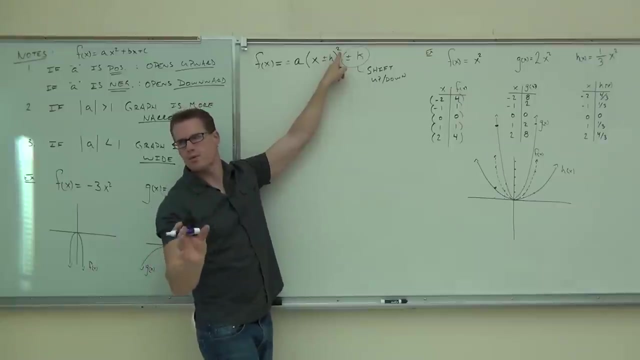 This is going to tell you whether you're moving up or down from the origin. That's what it says. Of course, plus means up, minus means down. here That tells you you're dealing with a parabola, but don't worry about that. 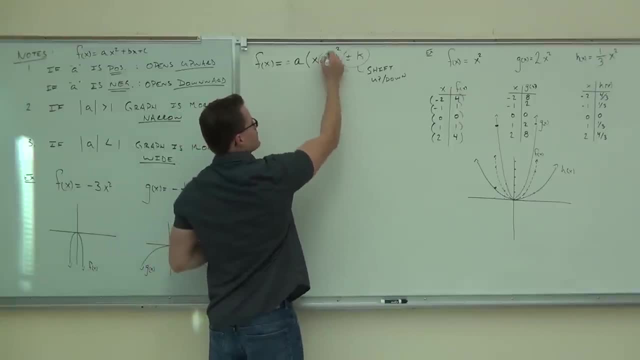 We're dealing with parabolas, this whole entire chapter, so that's automatically there. This plus or minus h inside the parenthesis there that says that you're going to be speeding up or slowing down your function. that means left to right shift from the origin. 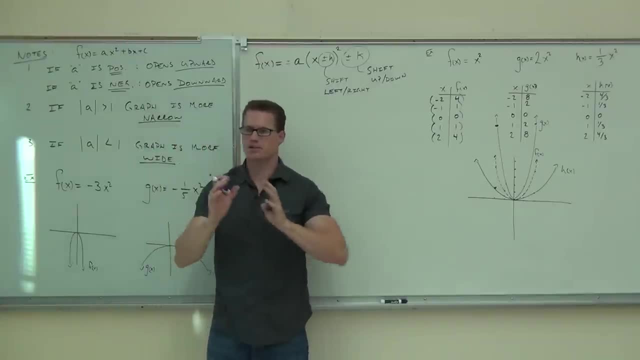 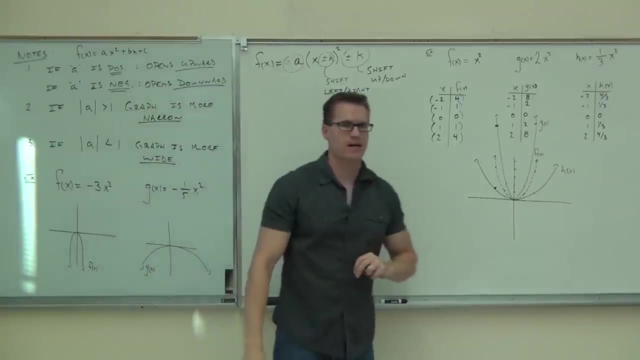 Of course, in this case, plus means left, minus means right. The thing that we haven't talked about until today is that plus or minus, a out in front of that, or positive or negative, Positive or negative a really in this case. 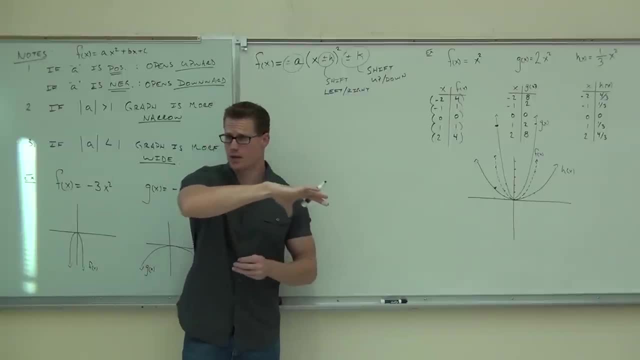 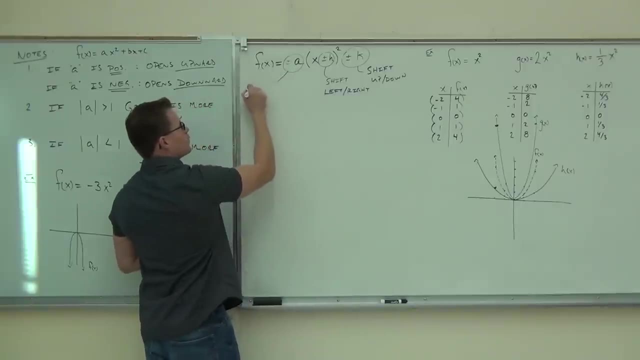 Positive means upward facing, Negative means downward facing. You had that already, but the value of a is going to tell you whether you're wide or narrow, so it does a lot for us. So here this is going to say one: upward facing or downward facing. 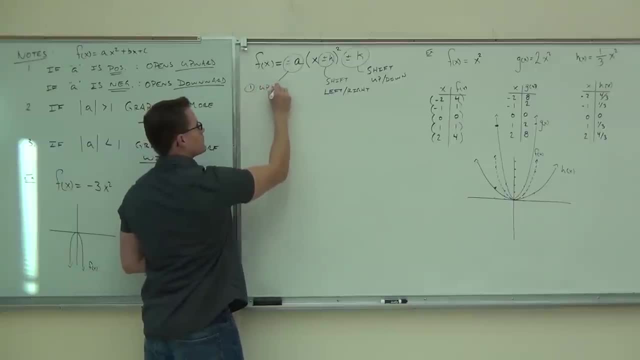 Positive means up, negative means down, Or opening, if you'd like to say that. And number two: it's going to tell you whether you're a wider graph or whether it's a narrower graph. 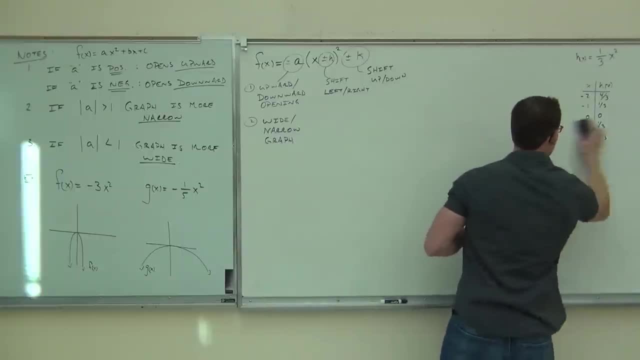 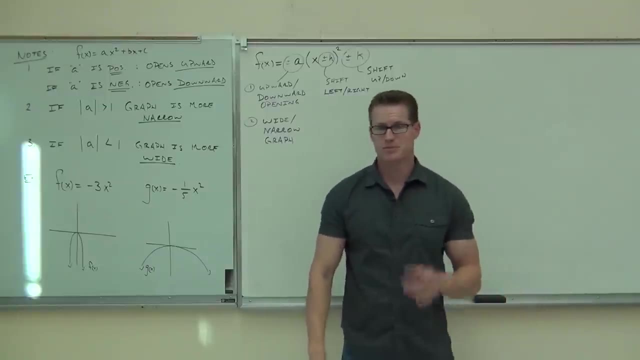 Two examples. We'll do one together. I'll give you one on your own. 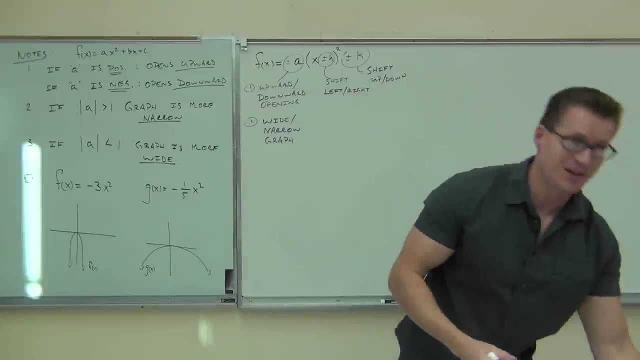 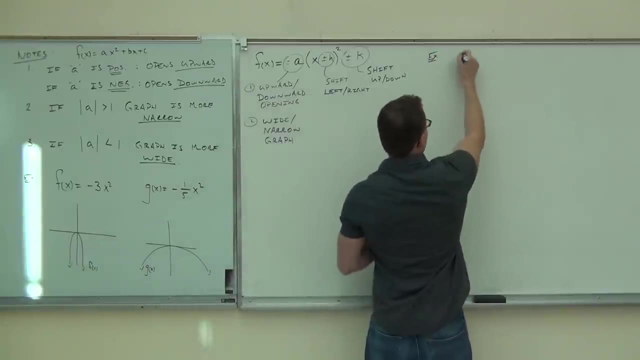 And that's pretty much it. I mean, we've conquered most of this stuff already, so it's kind of nice that we've done that. So I'll show you exactly how I want to see it. You're going to have a problem that looks very similar to this. 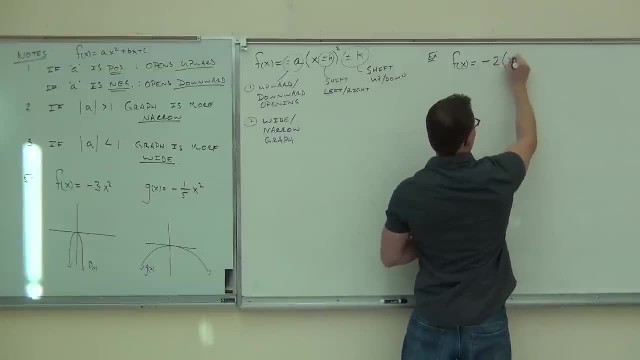 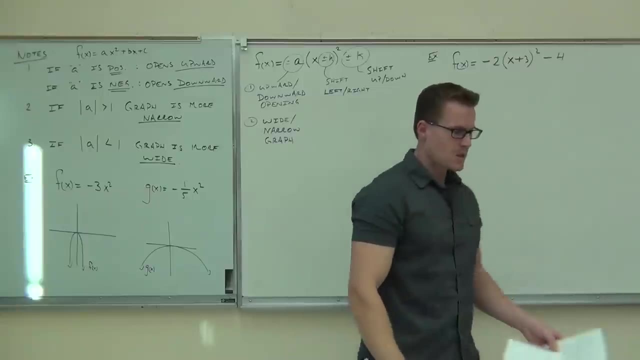 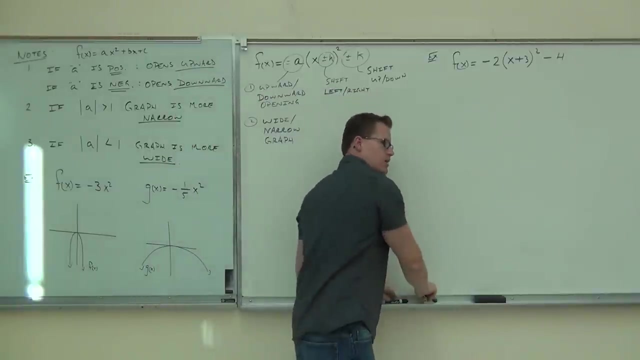 You'll have something like negative two x plus three squared, Let's do minus four. What I'd like you to do first is identify every piece of this, whether it shifts it or makes it narrow or wide, and reflects it or makes it upward, downward, facing. 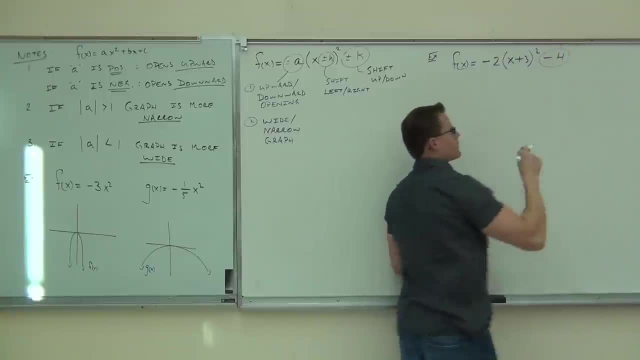 So we're going to start with the right-hand side. I'm looking at this minus 4.. Here's how I'm thinking about it. I'm thinking at the very end of my function. the only thing that I can possibly do it's. 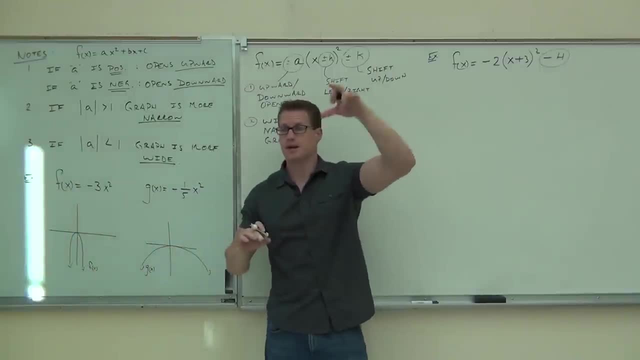 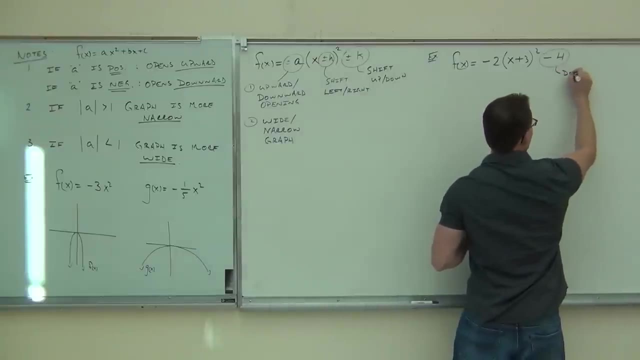 not in parentheses- is: move it up or down. I know that plus means up and minus means down, So that right, there is a downshift from the origin of four units, So I'll put here down 4.. Now I move on. 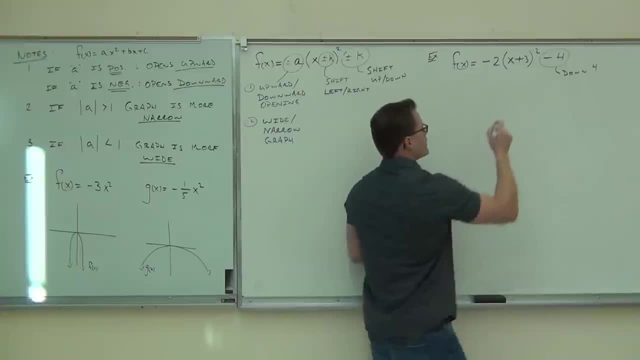 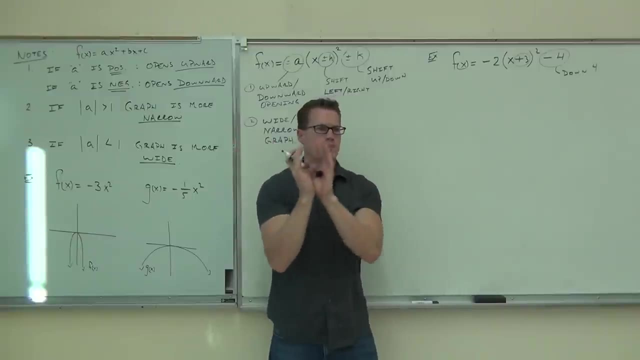 I know that x squared, That's verified. Then I'm dealing with a parabola. That's great. I'm going to go inside of my parentheses. I know inside my parentheses that speeding up or slowing down my function horizontally, So that plus that meant actually to the left. 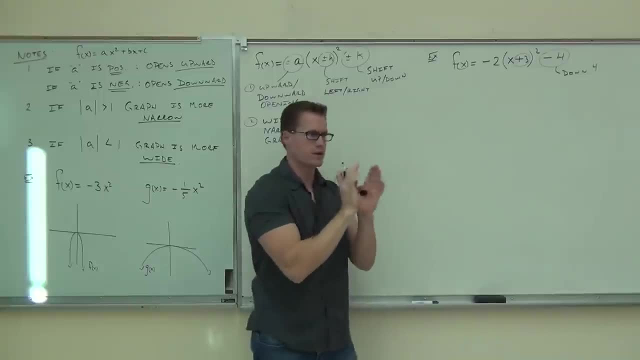 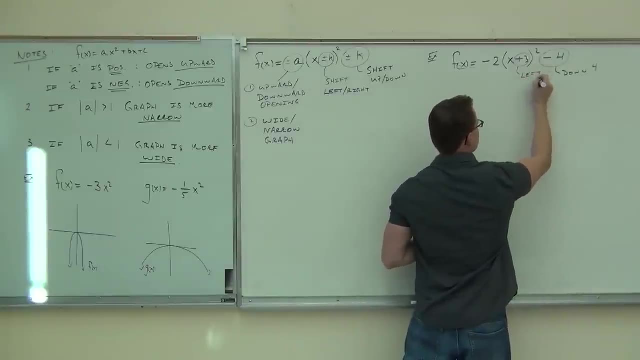 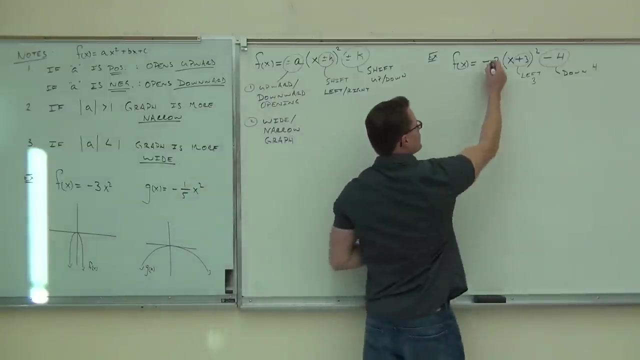 And the minus meant to the right. So get that straight in your head. what that does, This plus 3, is actually a left shift. Okay, Three spots from the origin. Now out here. this does two things for us. I look to check whether it's positive or negative, because that positive means upward facing. 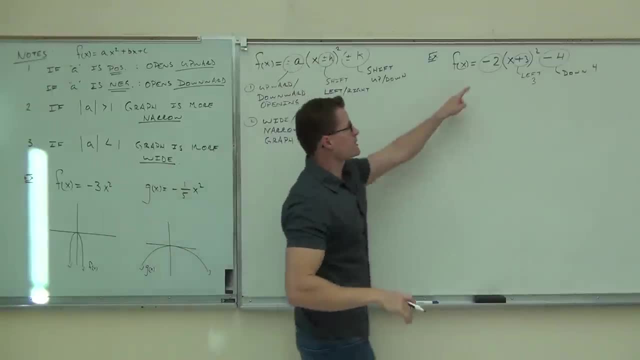 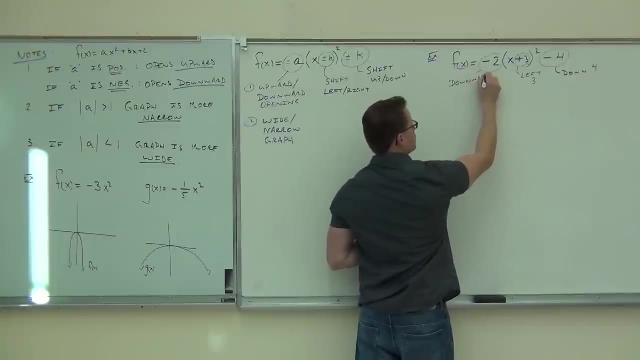 but a negative is going to mean downward facing or downward opening. This one is negative. So that means you're going to have two things going on. First, you're downward, Not shifting it down, downward opening. So I'll make sure I have that on there. 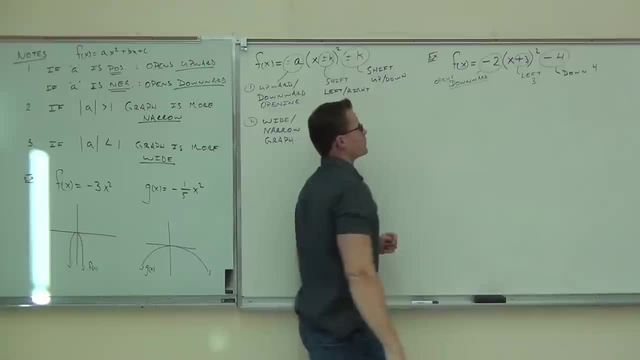 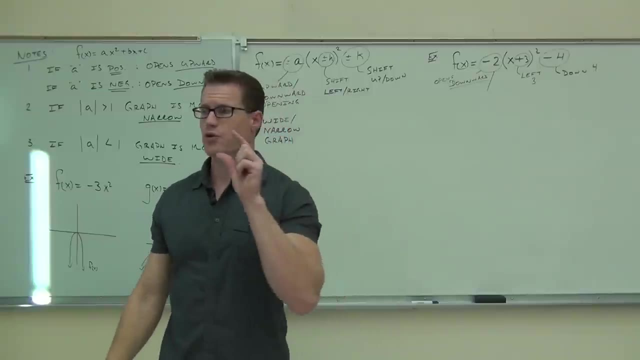 Okay, So it opens, opens downward. The other thing that does is it tells you whether it's going to be a wide graph or a narrow graph. Now, I don't consider the negative sign when I do this. That's why we have the absolute value over here. 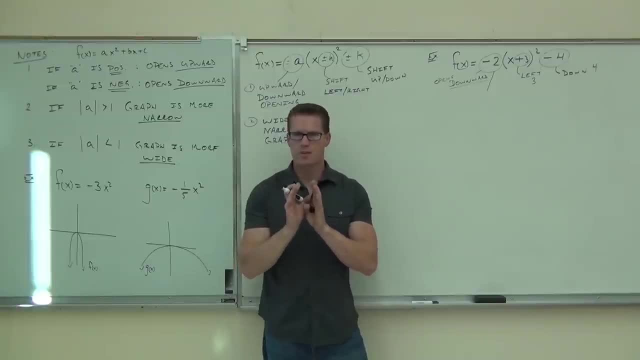 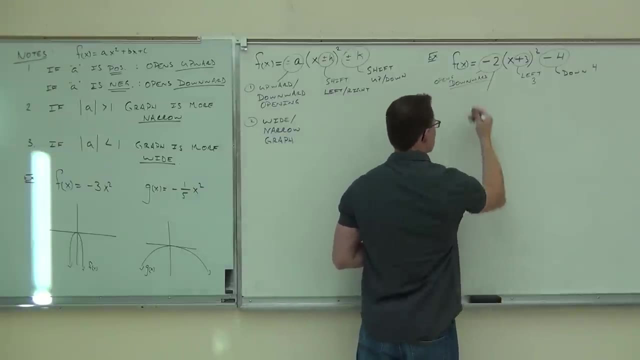 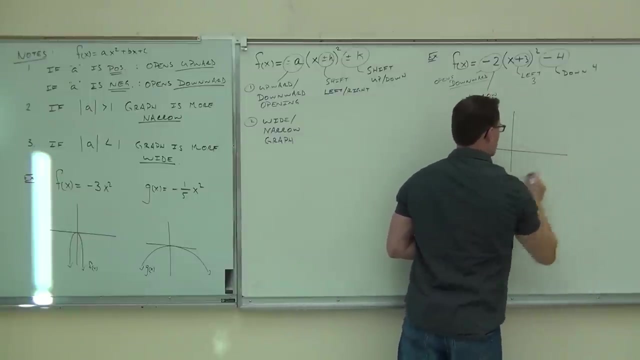 It says: you just look at that number 2.. That number 2 is greater than 1.. That means it's going to be more narrow of a graph. Okay, You can draw your original shape if you want to, but we all should know what that looks. 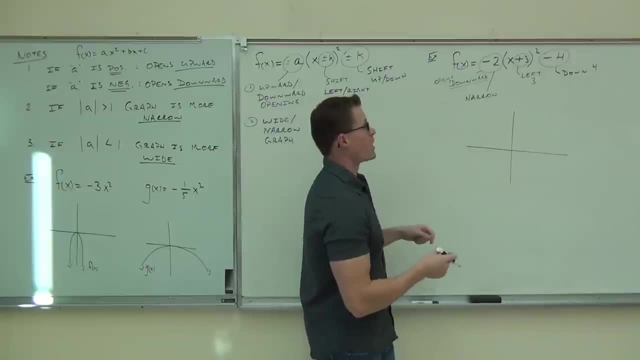 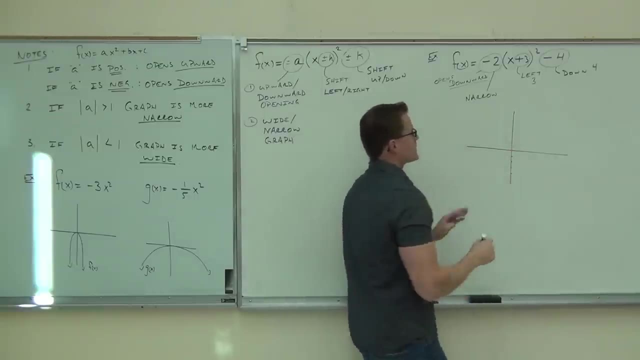 like at this point It's going to be our standard parabola. Then we're going to start shifting this around, So we start from the right to the left, just like we did up here. It says down 4, so I'm going to put 4 little hash marks there. 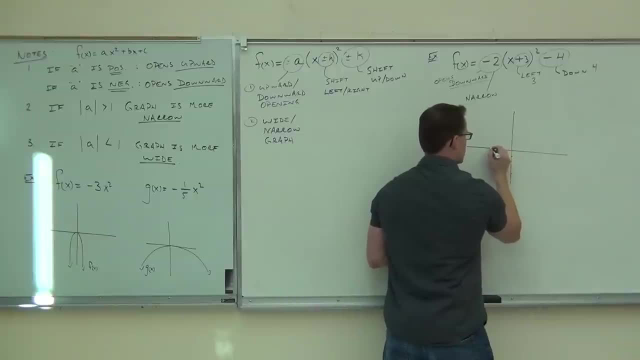 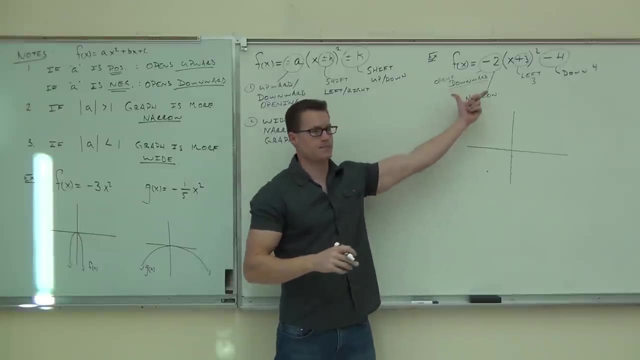 It says to the left: 3.. And that's where my point's going to go Now from here. this is where this kicks in. You've got to tell me whether you're upward facing or downward facing, It wouldn't matter, It doesn't matter. 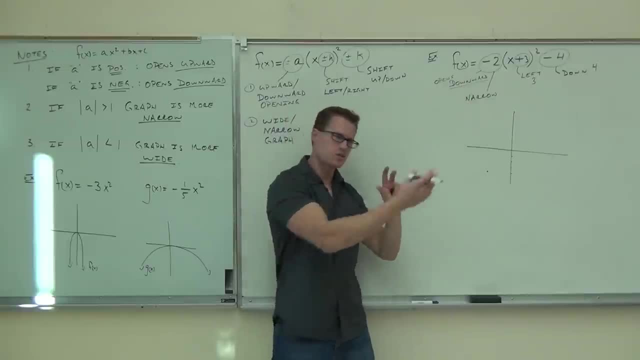 We've already done that. We've got to read what we've put out there. That's why I'm having to do it this way, so you can just kind of read it and be able to do what you already told me you're going to do. 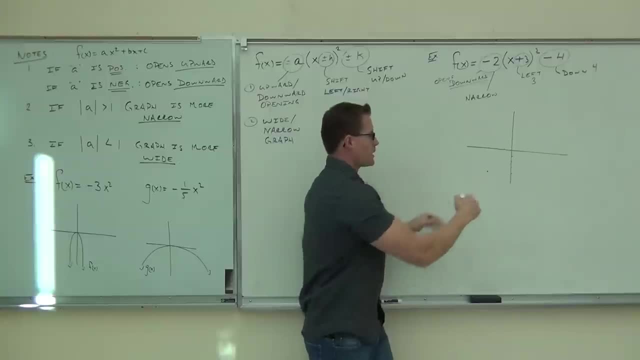 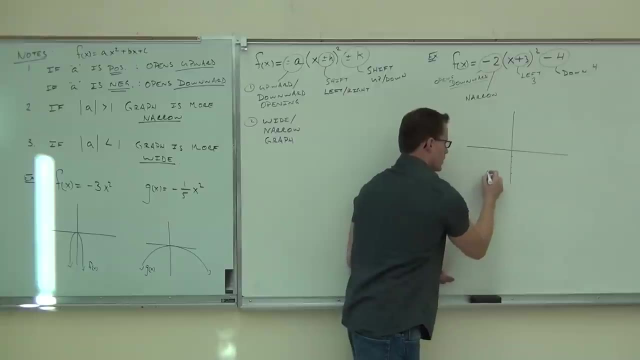 So downward, facing. instead of going upward, I'm downward and instead of drawing a nice normal sized parabola, it's going to be a little bit narrower. Now you're not going to be able to tell me exactly how narrow, because there's no other. 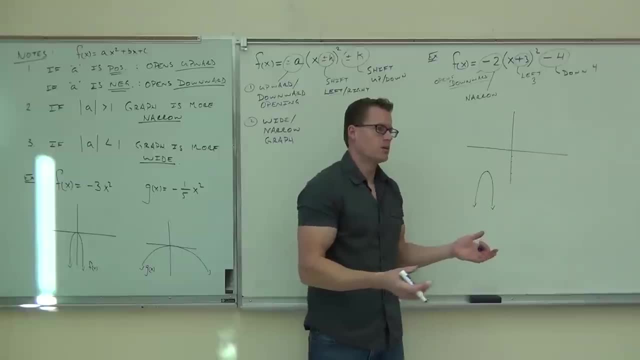 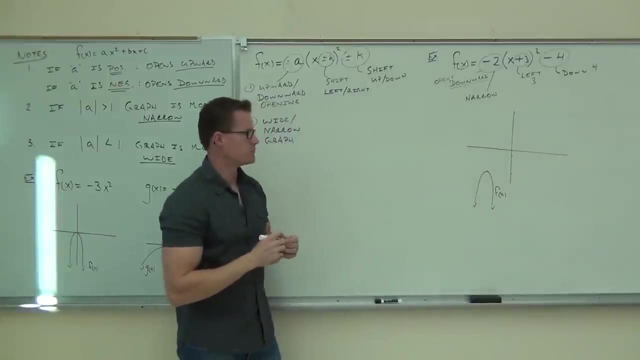 points. I don't want you drawing tables here. I want you estimating. We're sketching. That's why we can use all these principles here. Okay, Just make sure you're labeling it. That's your parabola. Would you be happy to be okay with this so far? 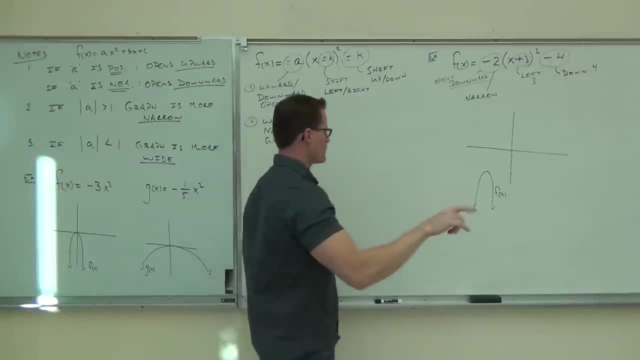 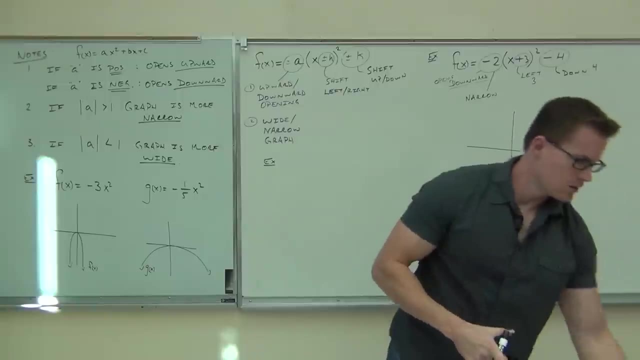 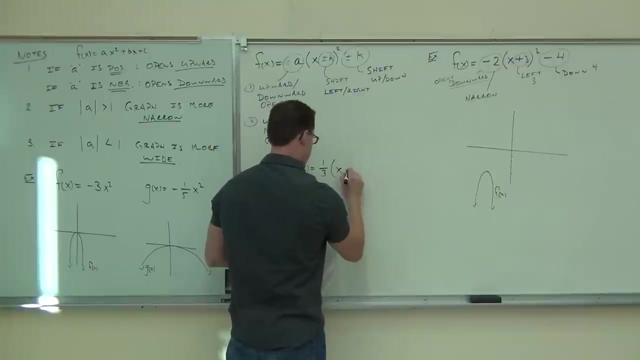 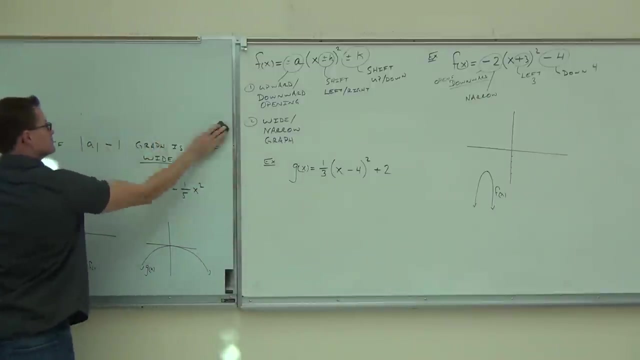 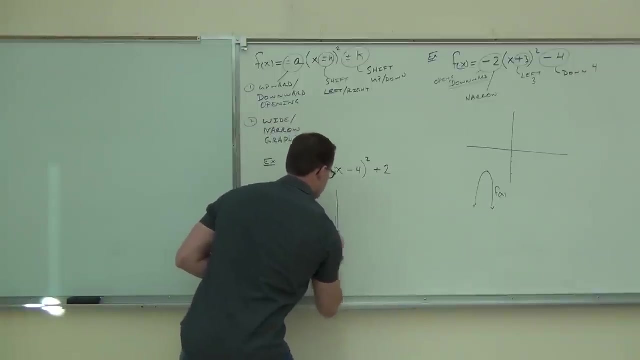 Okay, Let's do one more and have this on your own here. There you go, All right, See if we can get it. What's that piece? do somebody else. What is this piece? do right, right, very good, Okay, somebody else. 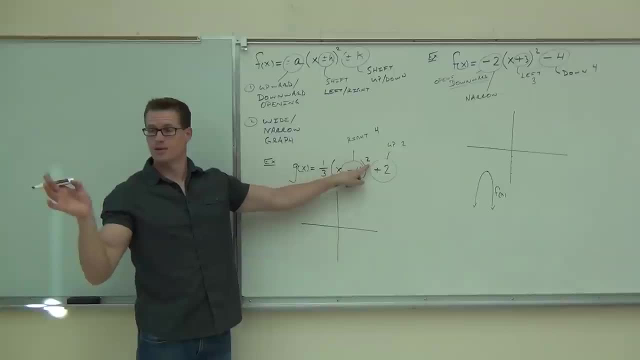 What is this piece do? Very good, and somebody else. finally, What is this piece do? Upward? very good, because why positive and wider? why The fractions less than one? so don't just assume, because it's a fraction, it has to be wider. 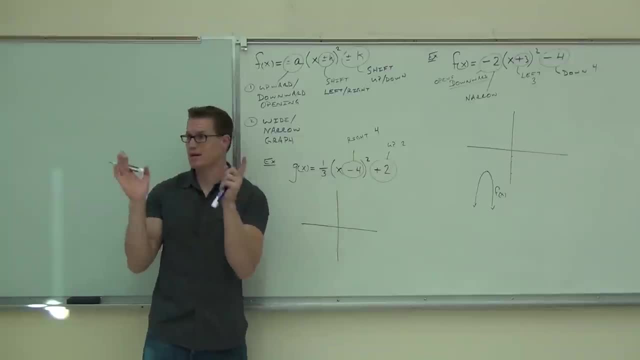 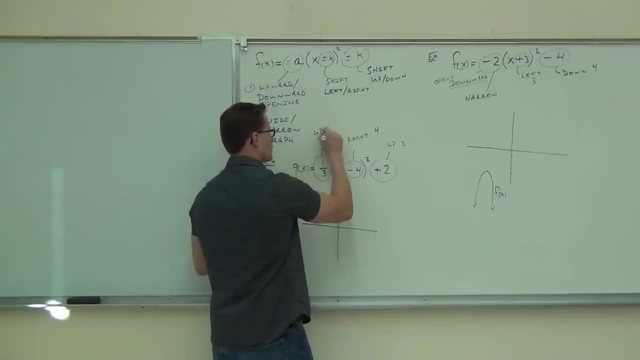 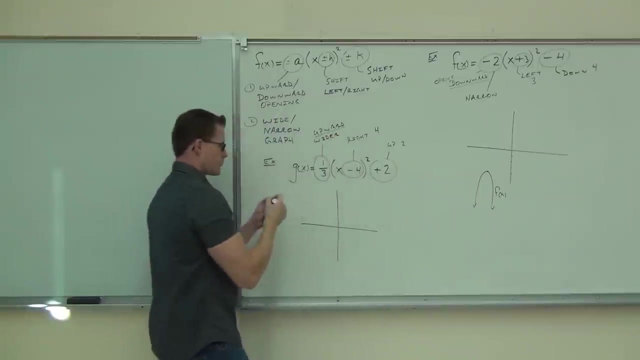 It's got to be fraction less than one. again. if I gave you seven thirds, that would actually make a narrow word. That's like two and a third I. So, from our origin, we're going to go up two spots. We were from right to left up two spots. 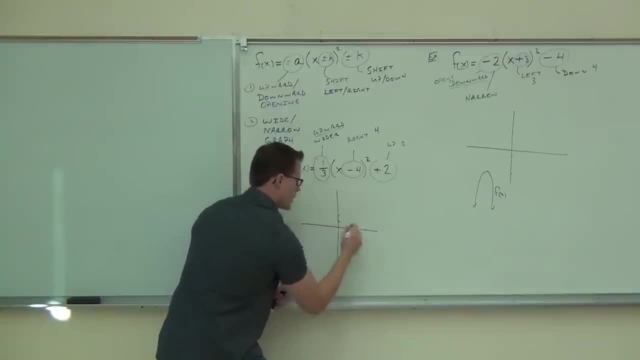 We're going to go to the right Four spots. We'll put a little dot there. It's going to be upward facing this time and it's going to be wider, so we're going to make a nice smooth, Wide parabola will label it. 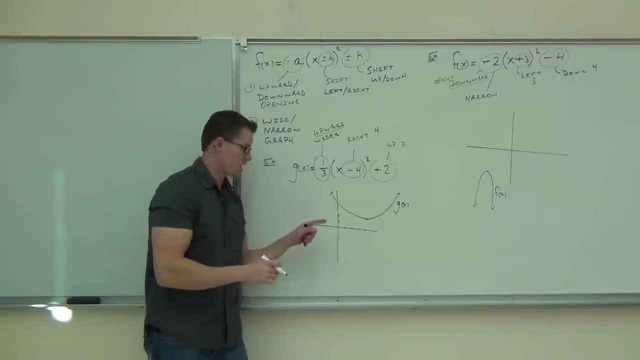 And that's about what you should have on your paper now. Do I know exactly where this cross of the y-Axis? No, I'm estimating. I'm estimating, but we're about to find out where that cross of the y-Axis. 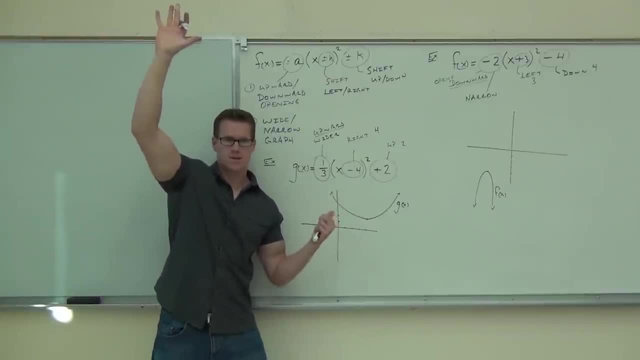 How much is that okay with what we've done and have that on the graph? Good good deal. Now I said we're about to find out where that cross the y-Axis, because we're going to do a little bit more on this stuff.